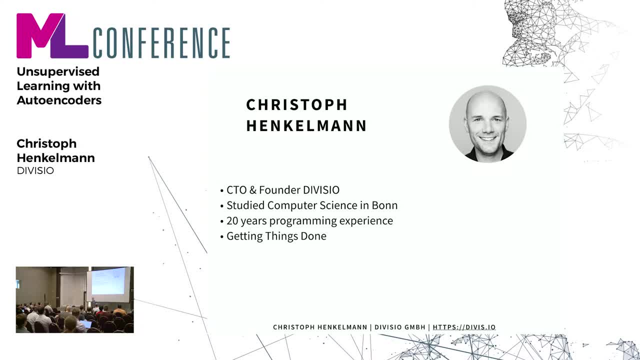 is nice and correct and proven well, But in the end, results count, So I have a more pragmatic approach. Yeah, My private Twitter handle is at C Henkelmann. The artificial intelligence stuff we blog and talk about is at Divisio AI. Yeah, So if you're interested in our blog and stuff, 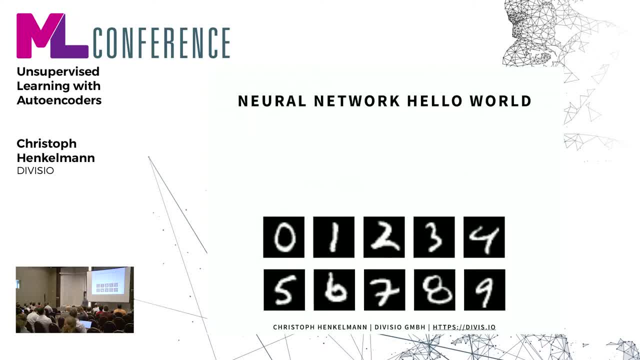 we write about, you can follow that handle. Okay, Before we get started with the actual topic, for some of you- maybe many of you- will know it, Some maybe don't, So I thought I'll quickly recap. We will work. We'll do all our examples here with a classic We'll. 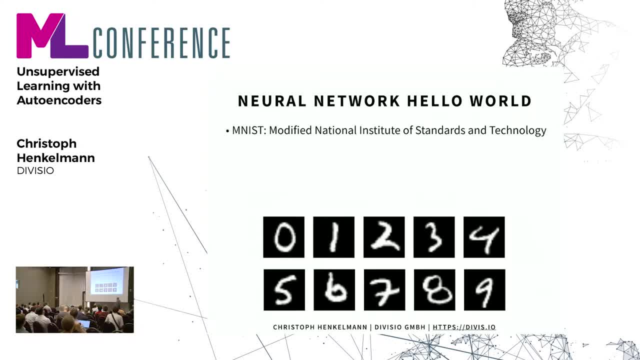 do all our examples here with a classic MNIST data set. MNIST stands for Modified National Institute of Standards and Technology And it's a data set of handwritten digits. So there are 60,000 training images and 10,000 test images. It's the hello world of neural. 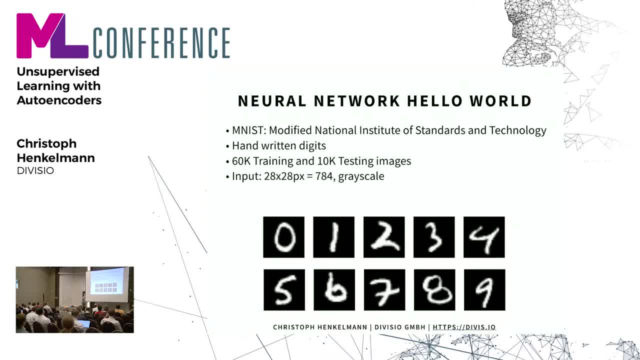 networks. Most of you will probably have used it already. I'm using it because everybody is so familiar with it And it gives quick results And you can actually do it on the laptop. So that was important for me in preparing this talk. So let's get started, Okay, So 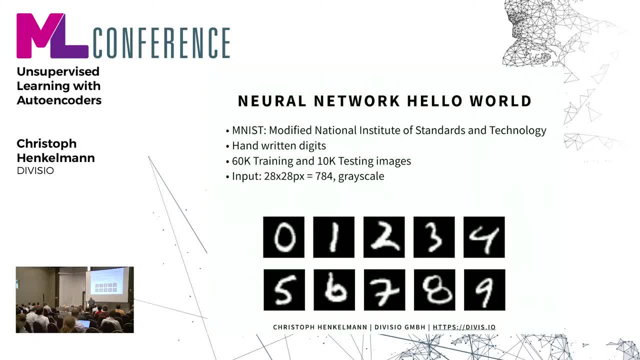 we have a lot of work. It's saved a lot of time that I couldn't do all the tests on the laptop. So what we have, the data set we will be using for all our examples will be 28 by 28 pixels grade scale images And they look like this, And mainly MNIST is used. 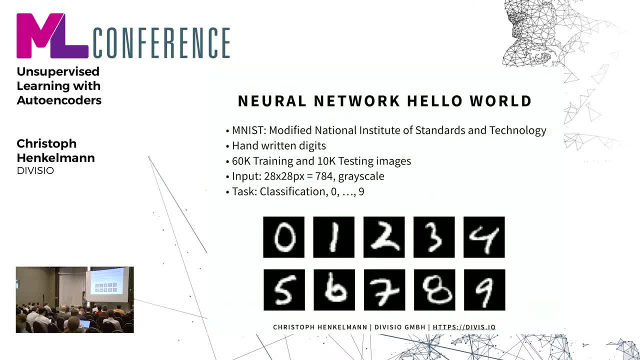 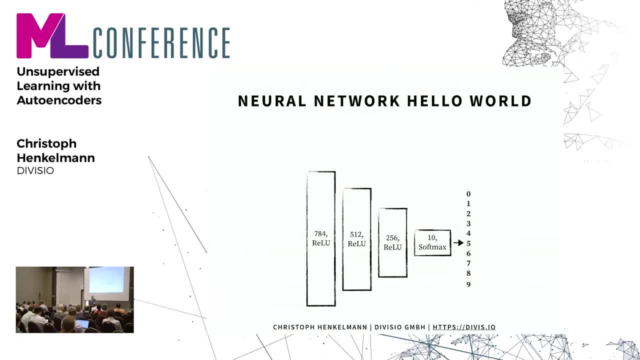 for classification, Obviously. It's to train a neural network to recognize digits, Obviously, And we have 10 classes, from 0 to 9.. And if you want to solve this, there's a very simple architecture. Many neural network architectures will solve this. The simplest one is a fully connected net. You can use it. You already get about 87% accuracy. 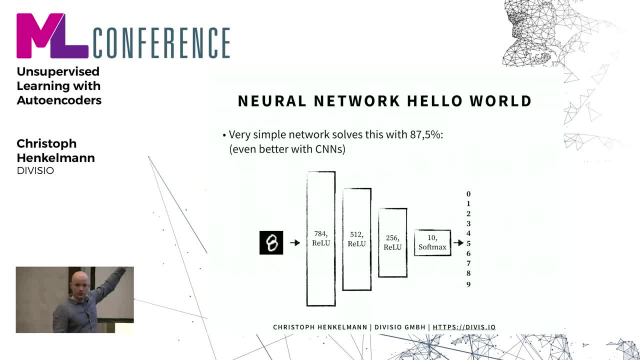 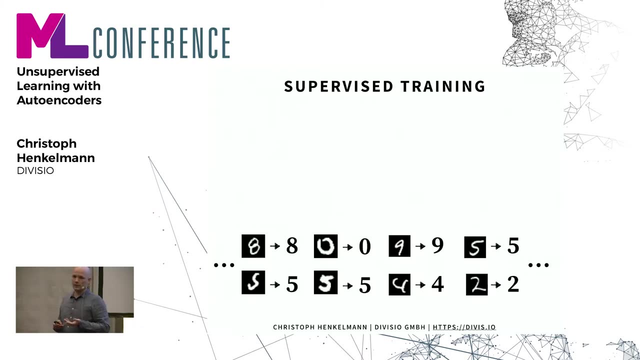 Works like this: You send in the pixels of our image into our neural network and then the neural network calculates the probability distribution. Why am I showing you this? Because this is a classical example of supervised training. Before we talk about unsupervised training, first I have to show you what supervised training is. 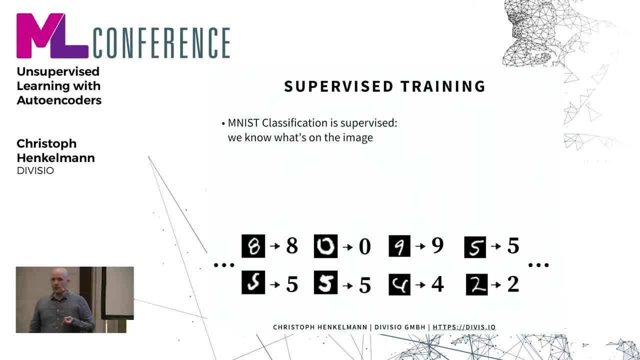 And why is it supervised? Because all those images are in folders and the first folder is named 0 and there are images of 0, second folder is named 1 and the images are of 1.. So we know ahead of time what we want to teach the neural network. We are the teacher and we supervise the training of the network. 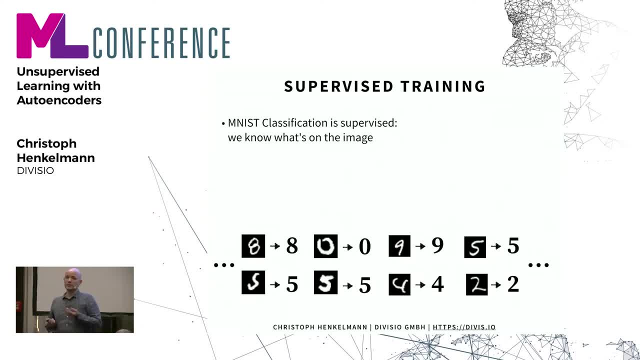 That's why most neural network on most ML is called supervised training, because we not only have the data but we know what is in the data, So we have to tell our algorithms what it's supposed to learn. Most ML you will encounter is supervised, like classification regression. There are many different ways of supervised training, but the principle is the same. 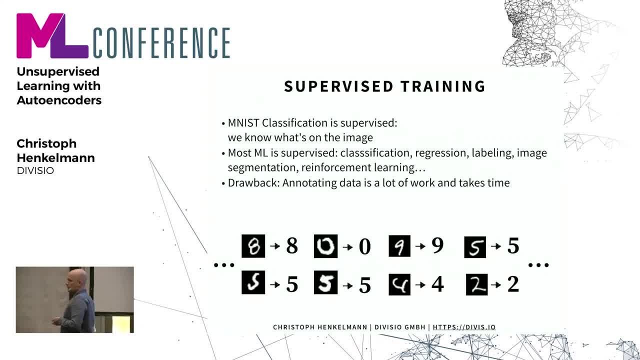 We have data and we know what we want to learn. There's a big drawback of that, and that is you have to annotate the data. MNIST is so useful and that's why I'm also using it, because somebody else has done the hard work. 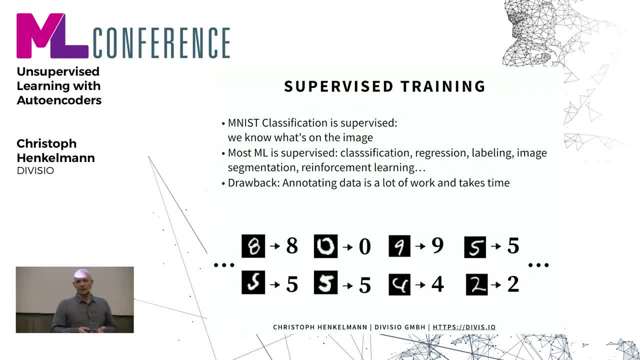 Somebody else has taken all those images, cropped them, centered them And has looked at them and has sorted them into the classes. And this is something that comes up in many talks here at the conference- that the data is actually the big problem. Good data makes good models, and not only is getting the data a lot of work, then annotating it is even more work. 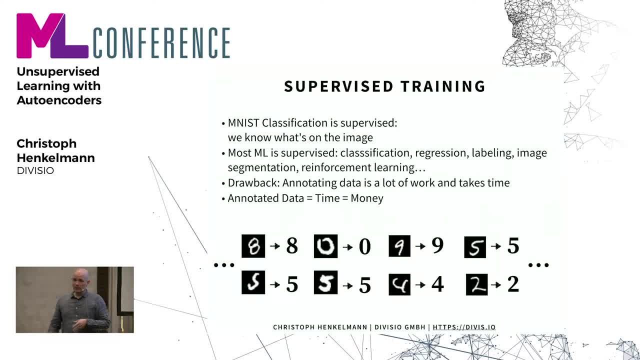 So I run my own business. I want to make money. at the end of the day, Annotated data takes time and we all know time is money. So if we don't, and also we need a lot of data and a lot of time means a lot of money- 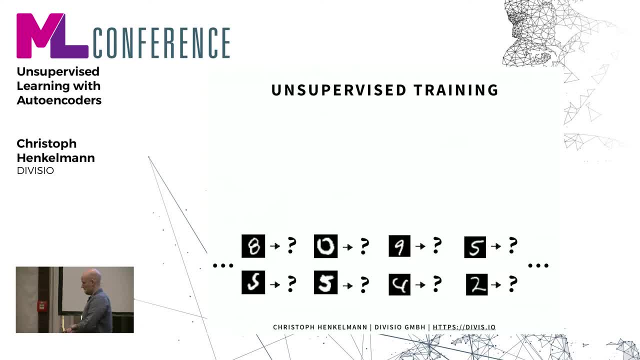 So there is unsupervised training. This is the other way to do things. Just imagine for a moment that we forget what is on these images. So we take all our MNIST images and we just throw them into one giant folder and we completely forget what's on the images. 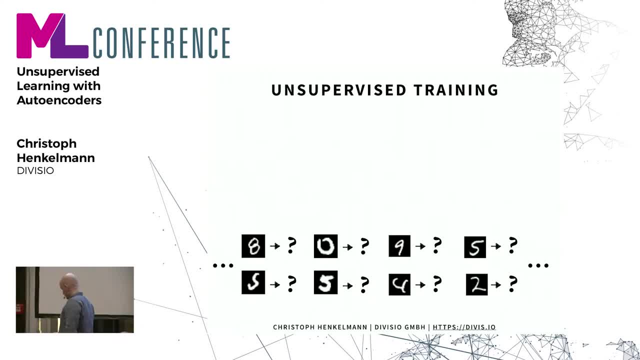 So is MNIST still useful for learning anything? Yes, because then we use unsupervised learning, As the name implies. we still need data, of course We need something to learn from. So unsupervised learning still needs data, But we don't need labels anymore. 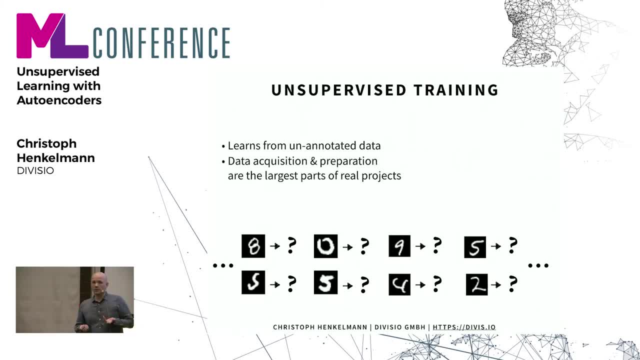 So, because data acquisition and the labeling is the biggest part in most projects. When we have working unsupervised learning, it makes our life a lot easier. But I mean, I can tell you this in advance- There is the famous no free lunch theorem. 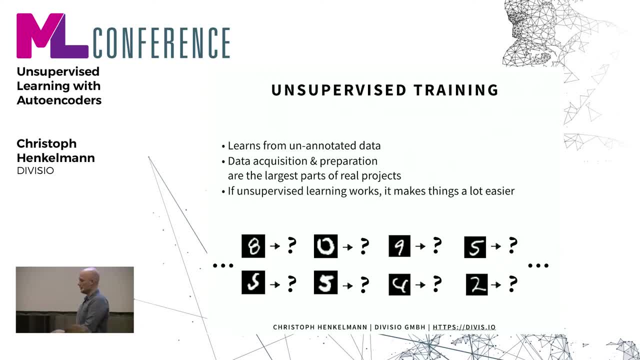 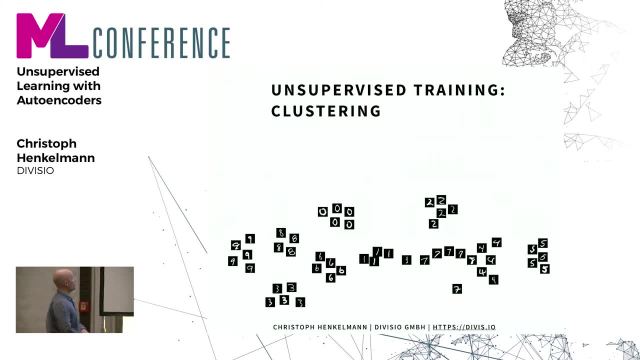 This applies here. It's not a magic. It's not a silver bullet that will solve all your problems, But it can be useful, as we will see later. Before we come to autoencoders, I will just quickly want to show you other kinds of unsupervised training. 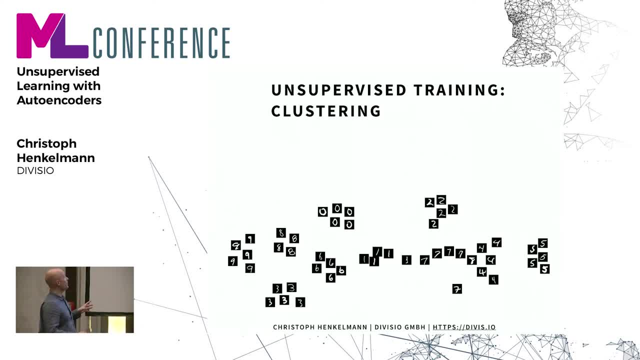 So you get the context we are talking about. The most famous example of unsupervised training is clustering. So imagine we have a. this, by the way, is a made up example to illustrate the point. But clustering would look something like this: A clustering algorithm would take the data. 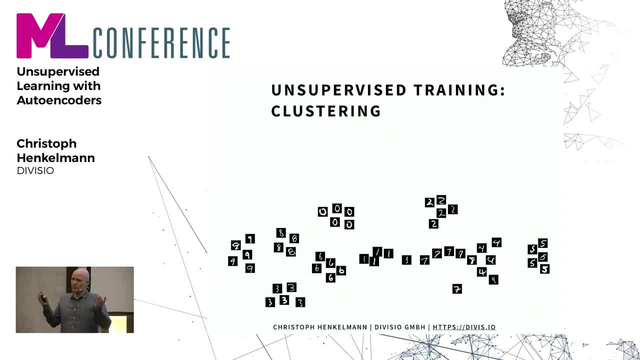 The clustering algorithm doesn't even know what's going on, What data it is. It's just some data, Some tens or some vectors. But what it will do? It will group similar data points next to each other And if we look at this, made up example, but it will work something like this: 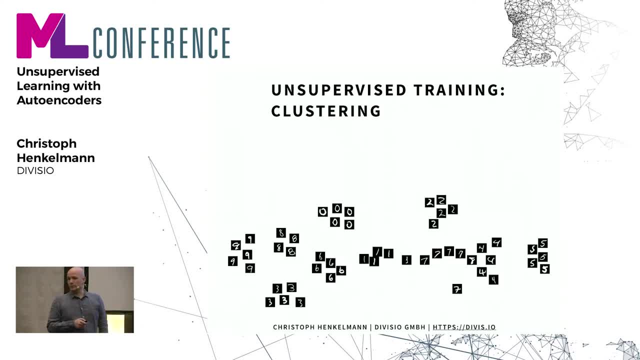 We can see we could actually use this as a classifier again, Because what you do is you cluster your data And you look at the individual clusters And, instead of annotating everything, you just look at some examples And you see: oh, this cluster is twos. 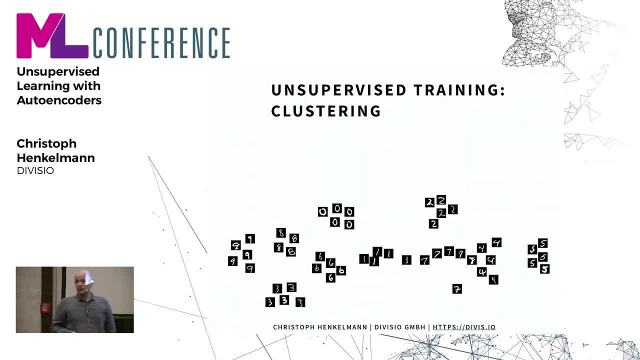 This cluster is zeros, And that way you can get a classifier Faster than annotating everything. There's a drawback, though. If you look at this, You will see here Is this a seven or a one, And these sevens slowly turn into fours. 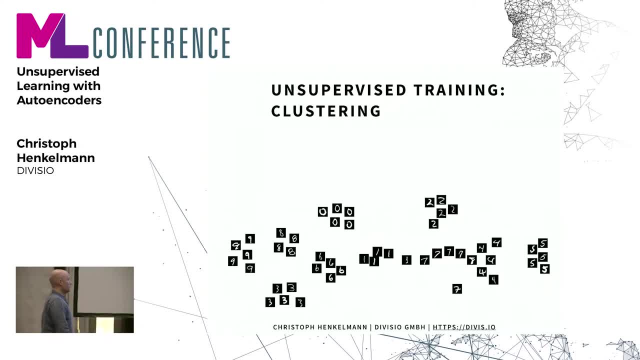 So clustering. This is a typical problem with clustering, That you have smooth boundaries. That can be a problem. What can you do with clustering? As I said, you can classify with it. Clustering is also useful, just for exploring your data. Just cluster it. 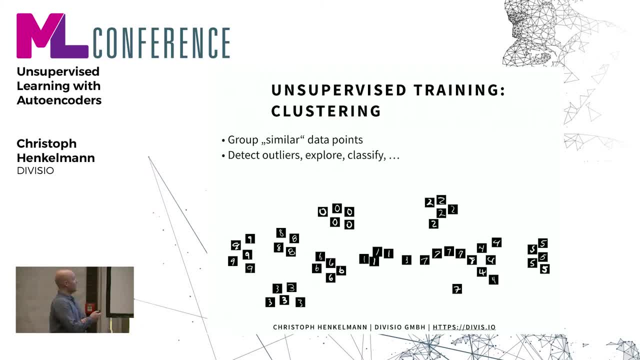 And look at the data And you will learn things about your data. And what's also very useful about clustering is outlier detection, Because if everything is in nice clusters And suddenly you have an image up here That's totally unrelated to the rest. 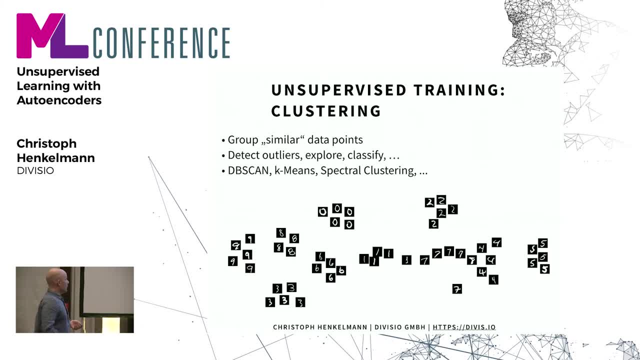 You know there's something dirty in your data. Typical methods include DB scan. K-means spectral clustering. But yeah, This is an interesting topic. I had another talk about this at the last conference, But we will stop here. This is clustering. 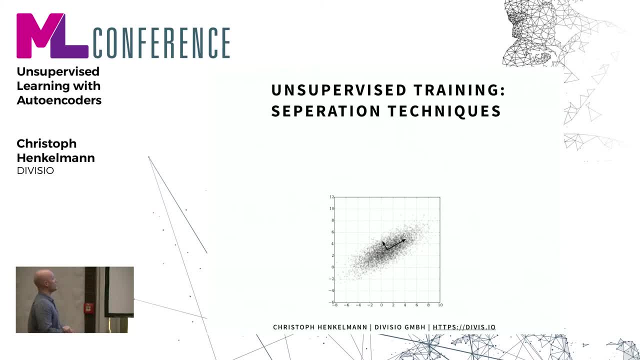 When people talk about unsupervised learning, It's mostly about clustering, But there are other techniques as well. I grouped them under the term separation techniques. That's not an official term, But these are techniques that are somehow related. All these techniques do the same thing. 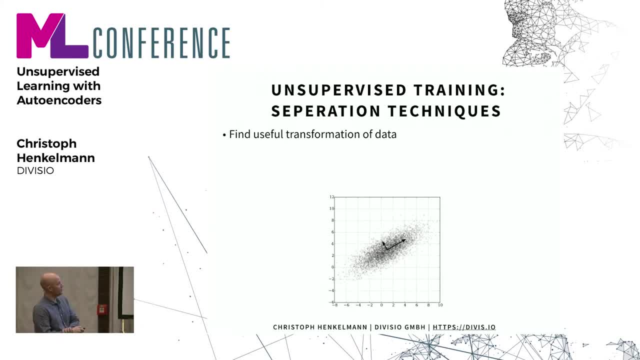 They find a useful transformation of data. I have this example image from Wikipedia. Oh, I forgot the image annotation I have to edit. This is just a Gaussian distribution of points And we can see here that it's not totally random. It has a certain direction. 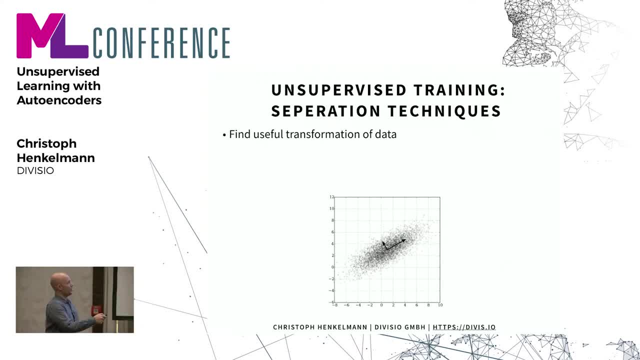 And we see that this direction is more important than this one, And this is something that these techniques do. They find important dimensions in your data And this can help you in understanding your database better. Say, you have data that has 1,000 dimensions. 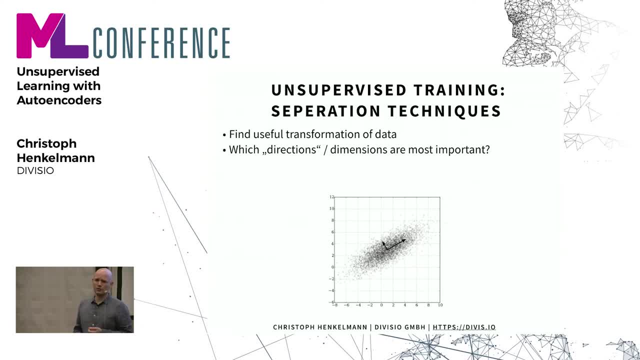 But you run one of these techniques And it tells you only three of them are actually important. Then you know something about your data. Again, What you can do with this is outlier detection. Very useful is you can use them to reduce the dimensionality of your data. 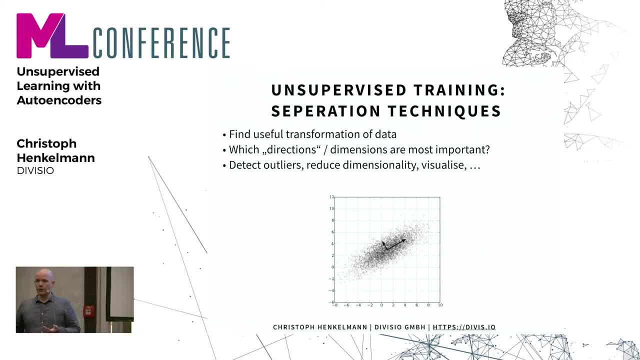 So sometimes you can use these techniques as a pre-processing step. Throw away dimensions And then your neural network has to learn less. Less dimensions means faster. convergence Means often better results. Typical examples are PCA. This is the example SVD, which is closely related. 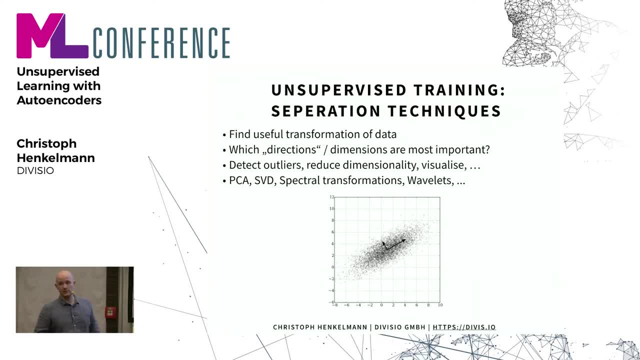 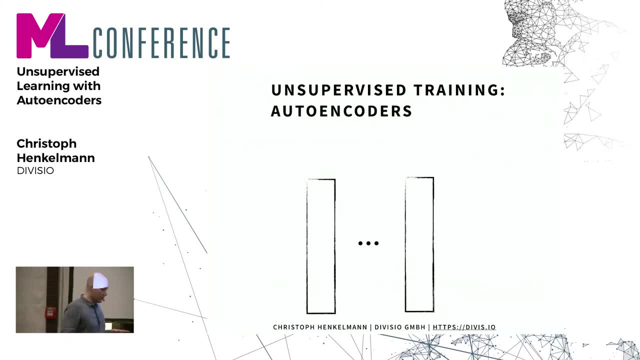 Singular value, decomposition, Spectral transformations, Wavelets. I grouped them here, Not technically correct, But from a practical standpoint these are somehow related. So let's get to the actual topic. A third kind of unsupervised training is autoencoders. 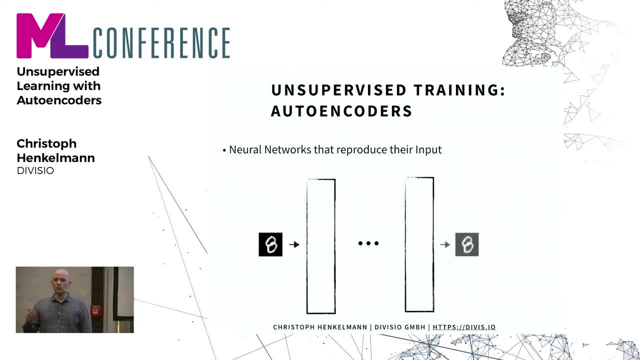 So autoencoders are neural networks that reproduce their input. So what happens is actually very boring. You take your input, You send it into a neural network And you get the same output I left. the magic happens here in the middle. Basically, the input is always the same. 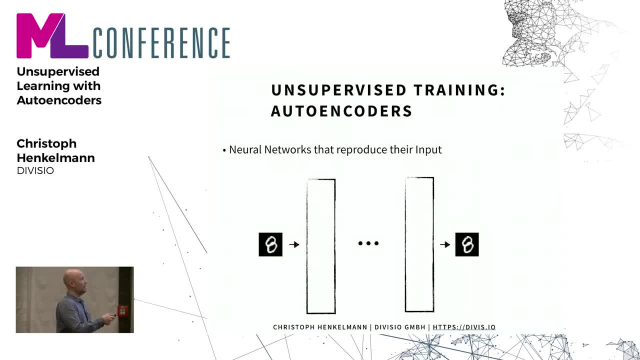 Of the same shape as the output, And here are all kinds of different architectures that we will now have a look at. In some way, you could say it's actually not unsupervised. Our annotation is the data itself, But well, that would be a bit technical. 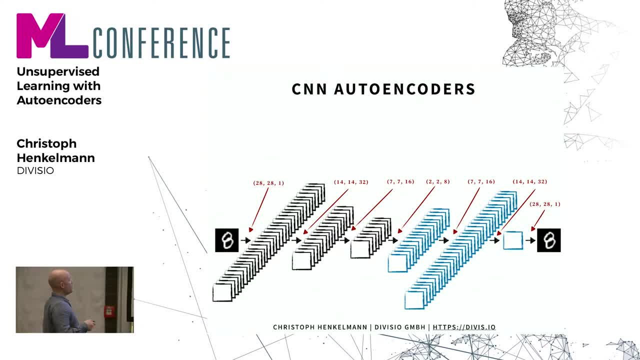 I have one example here. This is a bit more complex version of the net I showed you before. This is the one we will use to generate the images. It's a convolutional neural network. They are better at image tasks And here this is one thing. you just copy paste it together from some tutorials, tuned a bit. 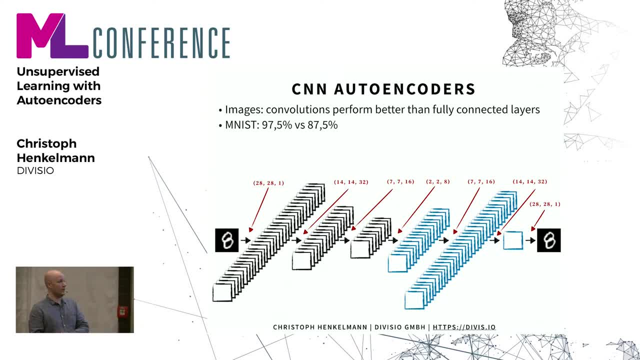 You can get like easily 97%, 98% on MNIST in half an hour on your laptop. I actually added this slide because when you use autoencoders and you work with images, You will need so called deconvolution layers, And everybody calls them deconvolution layers. 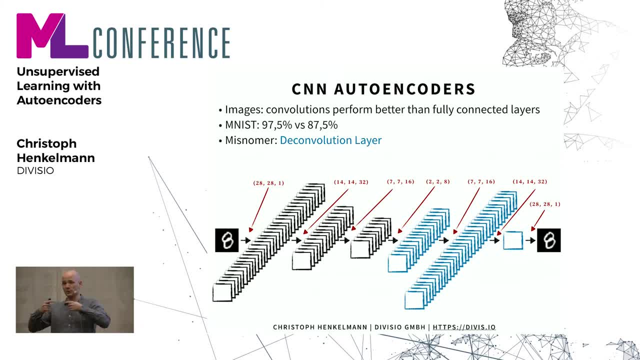 But I just wanted to make that sure, Because when you research it It can become confusing. They are often called deconvolution layers, But there is a mathematical method called deconvolution And this is not it. So actually they are called transposed convolution. 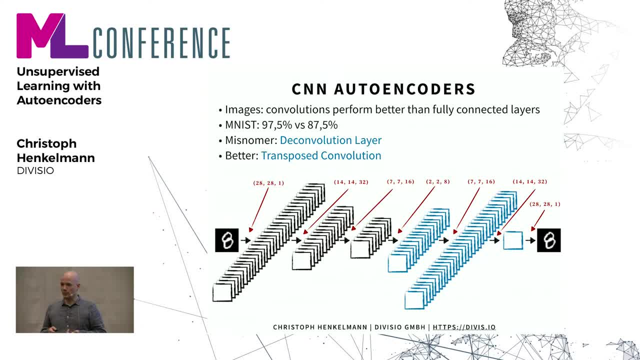 If you work with your frameworks, The frameworks do it correct. They call it transposed convolution, And when you try this for the first time, You open TensorFlow and look for a deconvolution layer, But there isn't one. So this is basically the idea of this slide. 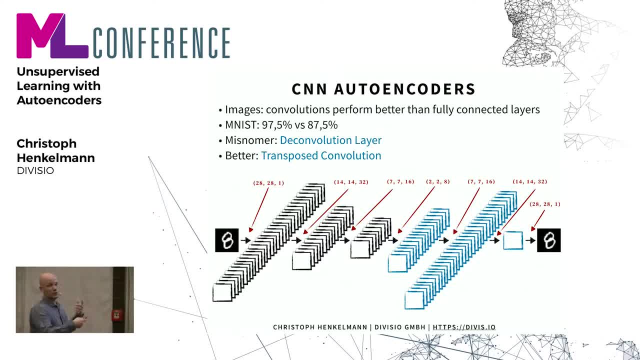 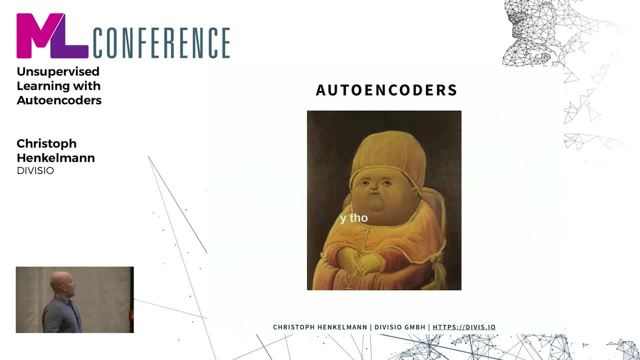 Transposed convolution is basically convolution backwards. We need to reconstruct our input, So we have to do the convolution step backwards. This is here in blue. Okay, And now you wonder Why, though? I mean, what good is it if I can reproduce my input? 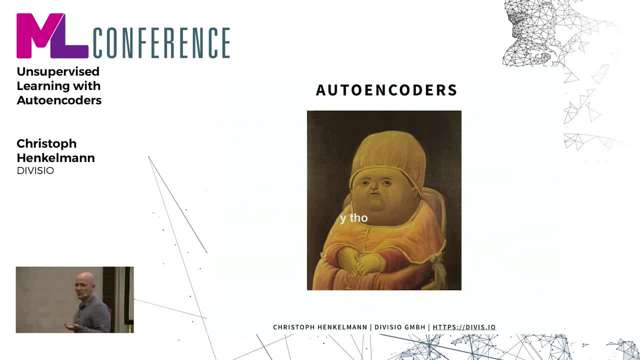 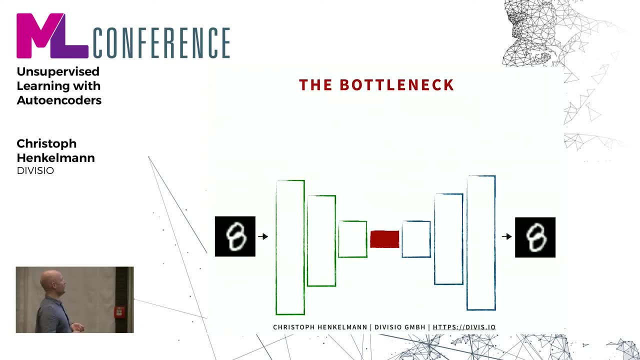 Right, I can do this without a neural network. I just take the input and output it, Job done. So why is this useful? There is one key idea For most autoencoders. This is why we start with it. It is the bottleneck. 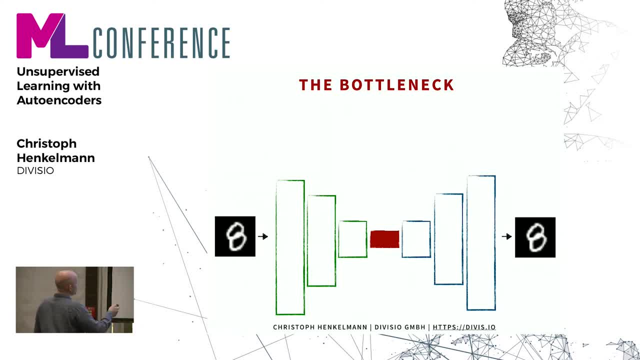 Here we see that our input is input here And our layers get smaller and smaller and smaller And here in the middle All the data passes through And then the network gets wider again. The bottleneck has a much smaller dimension than our input. 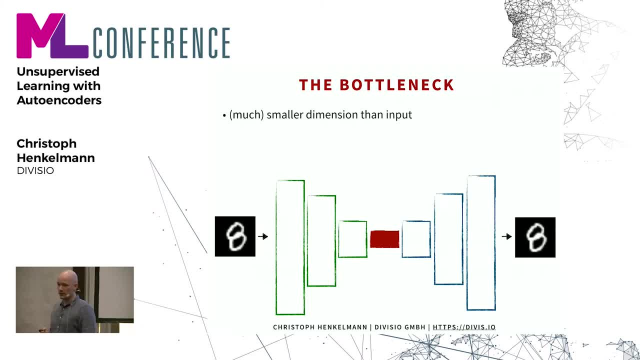 For our MNIST examples, The bottleneck has 32 neurons And MNIST has 786 inputs, So the neural network is forced to reduce the dimensionality of our input By a factor of a lot, So the net squeezes the information through this. 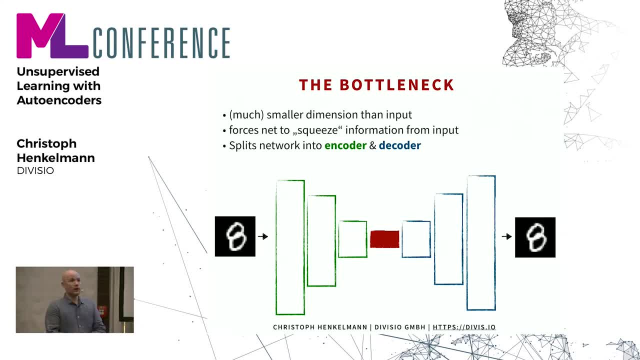 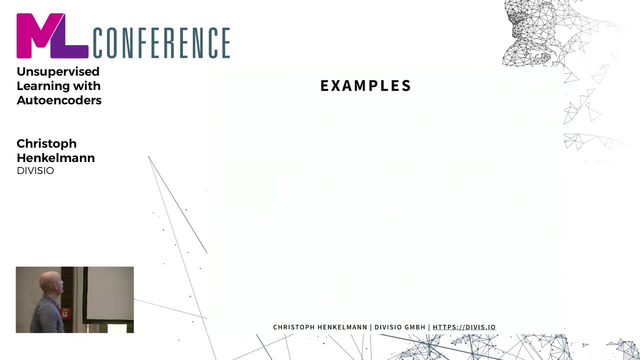 And this splits the network into two parts. The first part, Which feeds the data into the bottleneck, Is called the encoder, And the part that then expands the data again And tries to reproduce the input Is called the decoder. So let's look at some examples. 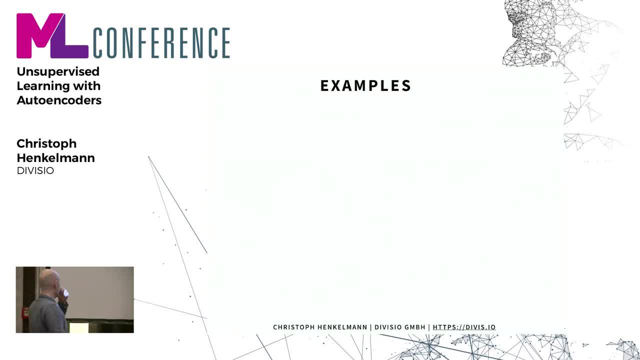 I did this with MNIST To make sure what I am saying here is actually all right. Let's look at some examples. I will come over here. It is better to show you. So this is the input image And this is what the autoencoder I built reproduces. 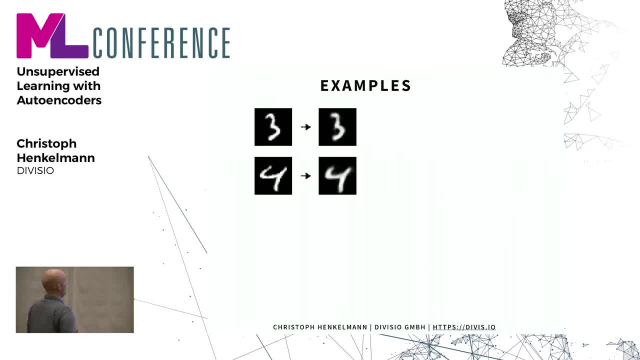 Okay, There is another input image, And here we see it is relatively well reconstructed. And another one, and another one. So it works. And again, you may ask why, though? Because what I actually built? Isn't this just a convoluted way to blur images? 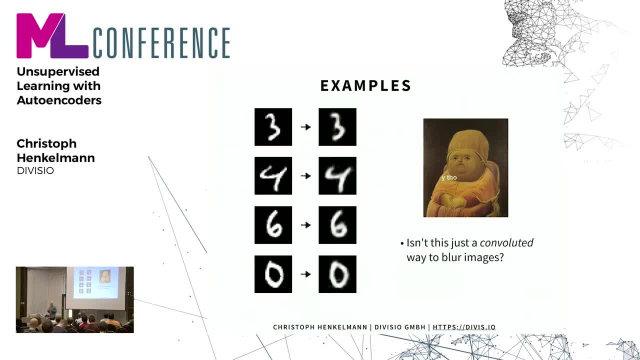 So we have put a lot of effort into building a neural network that blurs an image. We can do that with Photoshop or Gimp or whatever. But let's look at the data again, at some different data points. Look at this four, for example. 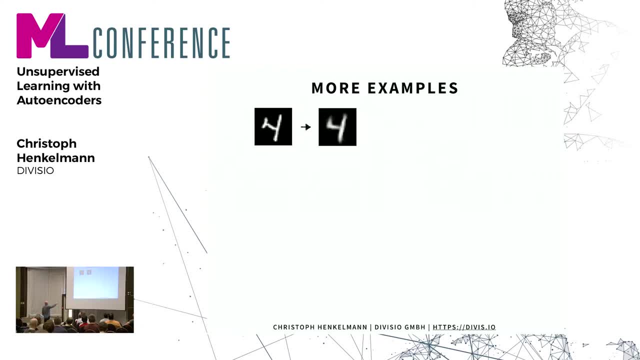 If you just look at it quickly You say yeah, it is blurred, But actually it isn't. You see here that the four has this little hook. It isn't present here. We see here that the zero is actually not connected. It is quickly written with a pen. 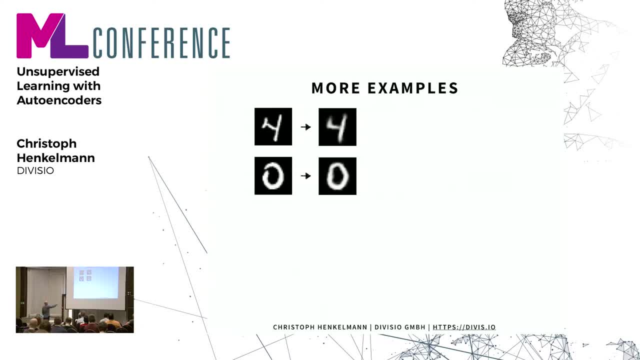 But this one is connected And it is not just the blurring. If it were blurred you would have some gray area here, But it isn't This. three looks the same at first glance, But you see that the lower part here is much longer here. 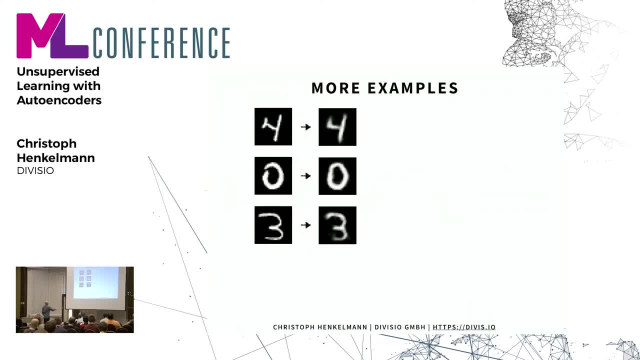 And here the upper part of the three is more curved Than this one, And this two, you see, has a much more curved upper part than this one. So we see, the images are not blurred, only They look blurred, But they are actually reconstructed. 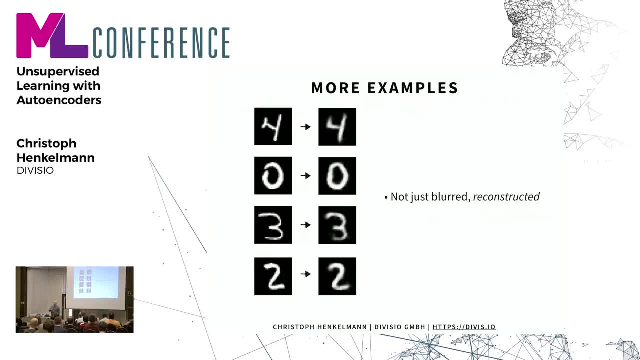 It is what you would do. if you quickly look at a number And I tell you to draw the same number, You would try to copy the style. If it is an American one, In Europe we do the one like this. In America they just do a dash. 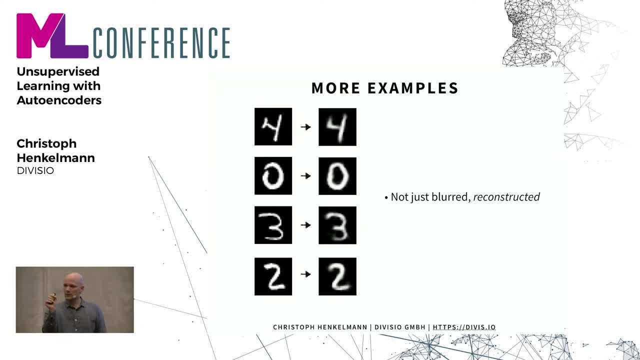 You would reproduce the one like that, But you wouldn't exactly hit it. You would hit the right positions, And this is what the net does: It reconstructs the input. Let's look at some more examples. Here we have what we would. 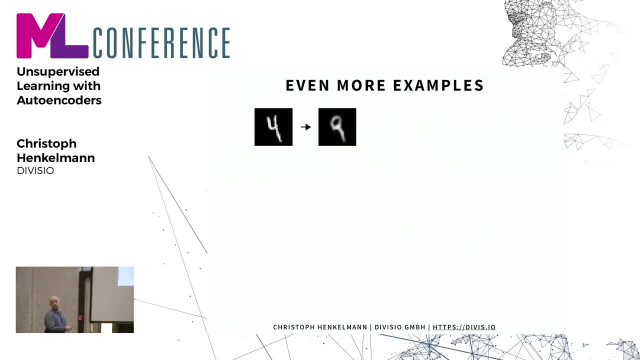 I hope everybody would agree, is a four. See what the network reconstructed. It thinks it is a nine. And this one is even more interesting. I would say it is a one. I am not quite sure, But this is more of a three. 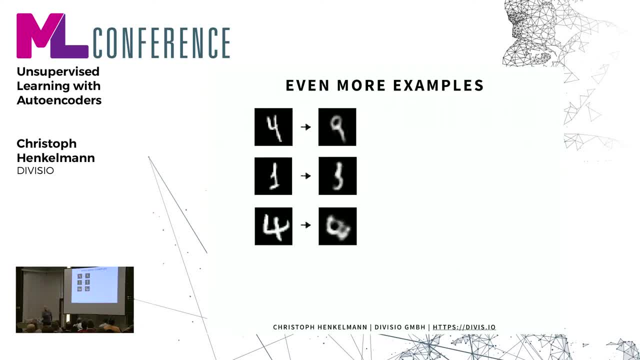 And we see that this looks quite different from this one, And this is even stranger. This is a four, But the network has a problem with a four With such a long dash, So it is just kind of like a squashed eight. 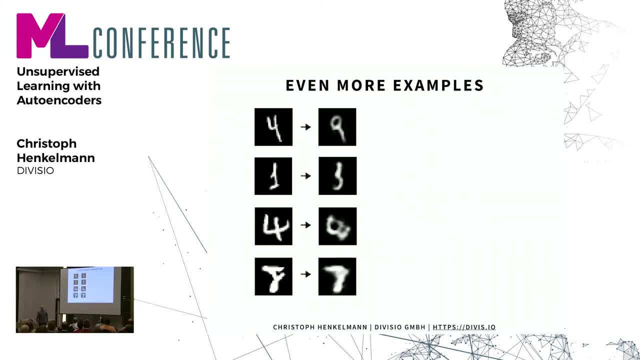 And I don't know what this is, But it just ends up in a blob. So what do we learn from this? Unusual images, Images that are not like most of the other images in the input, Get worse reconstructions, So the reconstruction isn't just blurred. 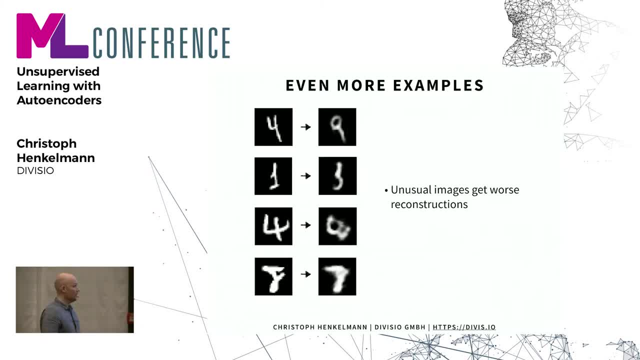 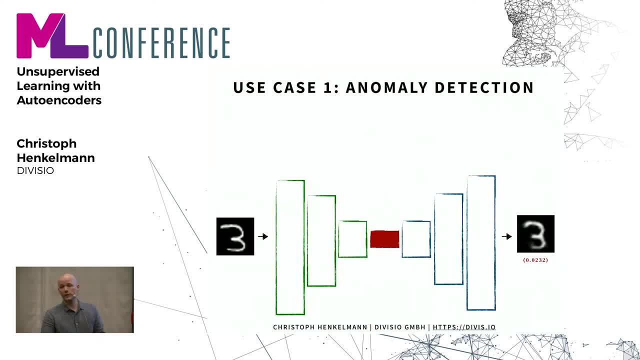 Or it is just simplified. It is actually wrong. So, with this idea in mind, We actually can build something, Something useful, of our autoencoder. Use case one: It is called anomaly detection. Sometimes, if you Google this, It is called the anomaly detection autoencoder, I guess. 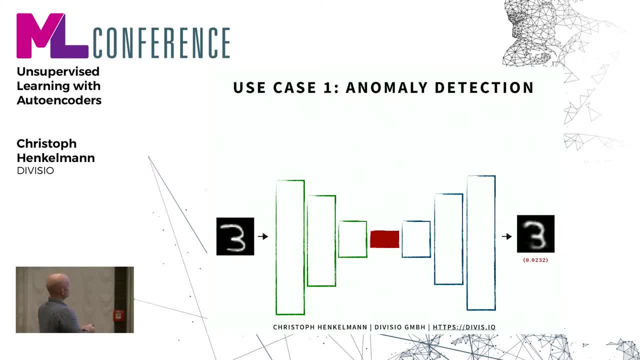 And what happens is We input an image, We send it through our network And at the end we get our reconstruction. But we don't only get a reconstruction, We also get a reconstruction error. Often L2 or L2 error is used. 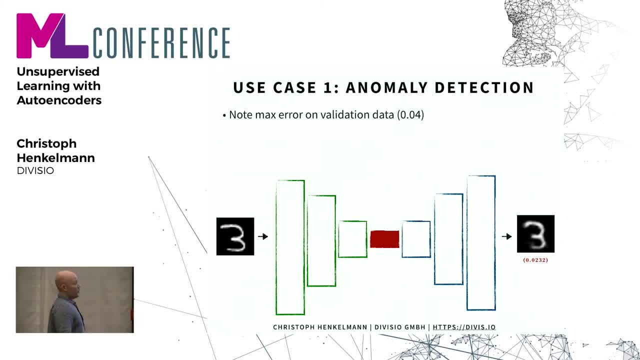 You can use all kinds of error measures, And, And what we do now is We take our training data, Our unlabeled training data, And just pump it through the autoencoder. Let it learn, learn, learn, learn, learn. 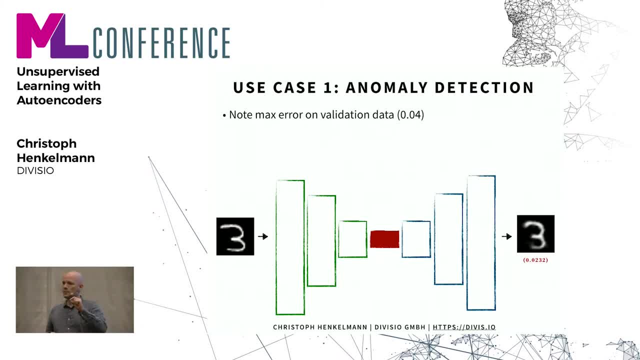 Until it converges. And then what we do is We note the maximum error We have on our training data. In the case of this MNIST data set, I had it 0.04.. So I just said okay, 0.04 is the worst case I encounter. 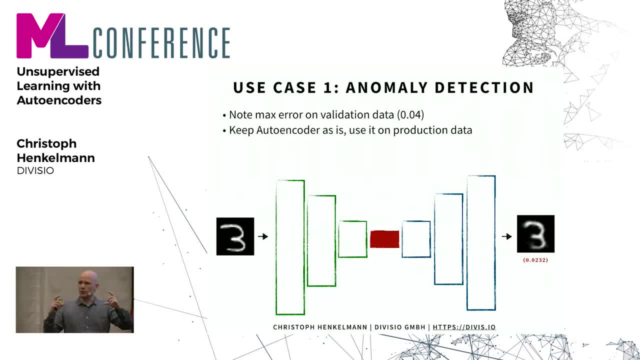 When I work with this. And then we take the autoencoder Just as it is And we take it into production And then We feed it real data That we encounter in production. And now what happens is If I encounter data with an error. 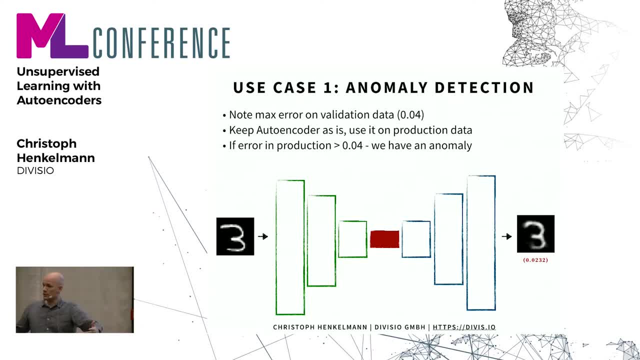 Larger than 0.04.. Because you know, in production There's an image we haven't seen before. The image is fed into our autoencoder, It gets reconstructed And we get the reconstruction error. And if the reconstruction error is too tall, 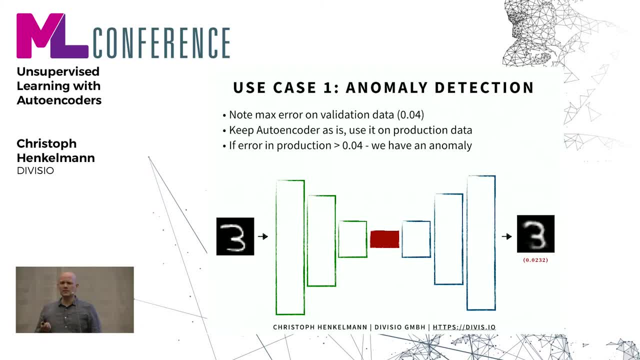 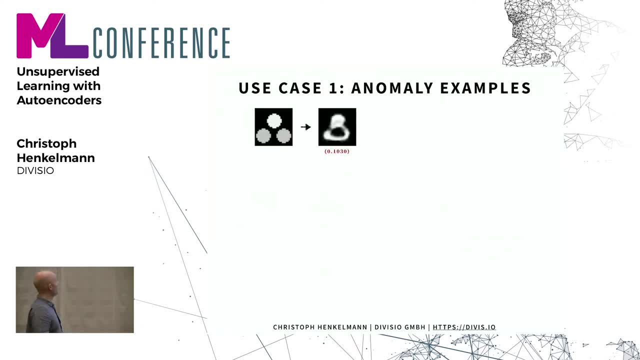 Too large. We say This is an unusual image. This is some kind of anomaly And let's try that. I made some images myself. I made this beautiful image here With GIMP And see Look at the reconstruction 0.1.. 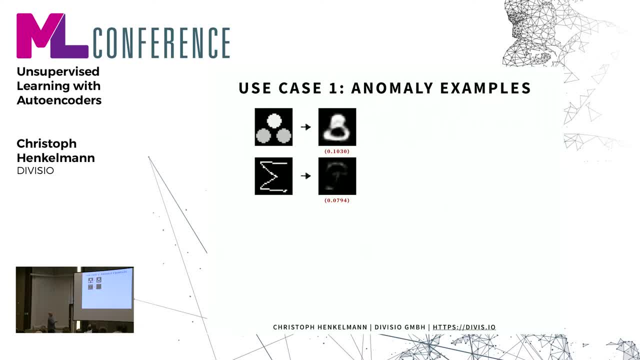 Totally broken. reconstruction. Added a sigma, Also broken. reconstruction Error of 0.07.. Added this little smiley, Also not properly reconstructed. So in just half an hour I built a network That can tell you If something is a digit. 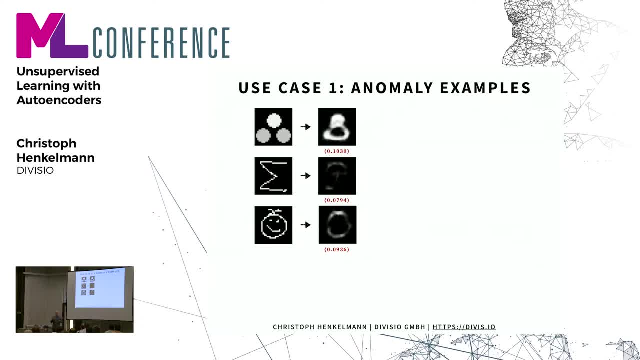 Or something completely different. Normally, if we build a classifier, For example, spam, No spam, You have two classes: The ones we are looking for And the anomalies. We need balance data. We need examples of what is right And what is wrong. 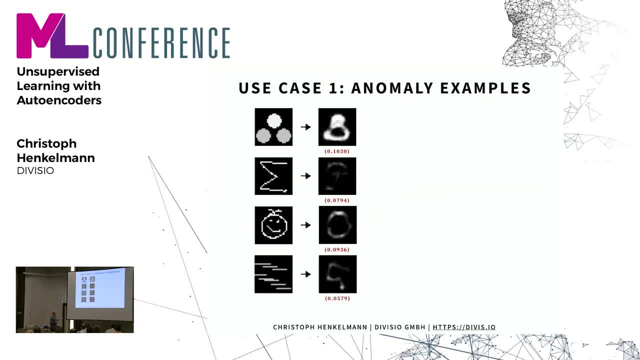 But sometimes in the real world- Oh there is another one. Some stripes Also gets badly reconstructed If we have unbalanced classes In the real world. Say you have a nuclear reactor. I mean, I am not suggesting nuclear reactors Should be totally controlled by ML. 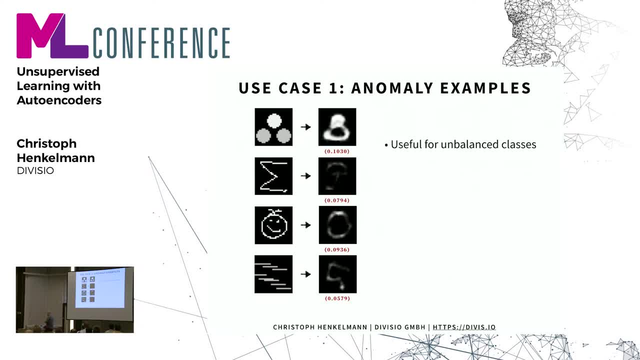 But it might help. The problem is With a nuclear reactor Is you have all kinds of pressures And valves And what not. It would be cool If you have an additional system That can control it, But it might not work. 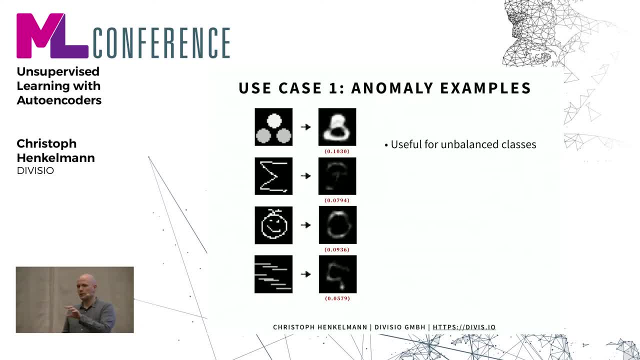 And it might not work, And it might not work, And it might not work. But if you have an additional safety system That tells you Something is wrong, You know, Like a good engineer When he hears a certain noise In an engine. 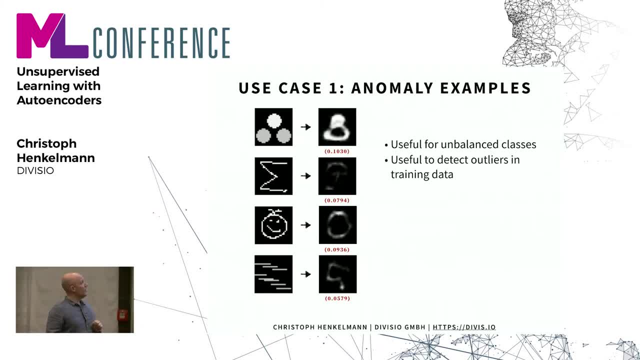 That he hasn't heard before. He knows something is wrong here, And the problem is We can't blow up a few thousand nuclear reactors To find certain configurations That are bad, Right, But what we have Is hopefully Thousands and thousands of hours. 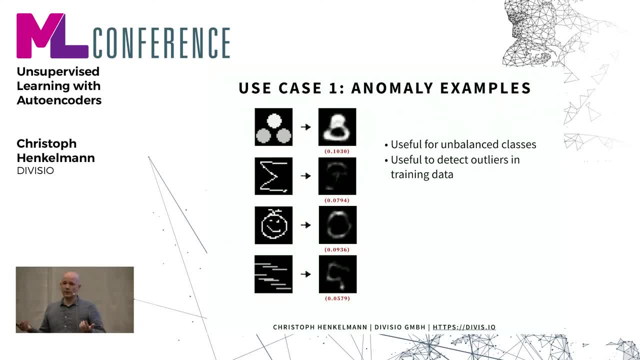 When these things run properly. So if you have got some kind of industrial application Or something Where a lot of data is created And most of the time Everything is okay, But you want to make sure You have an additional way. 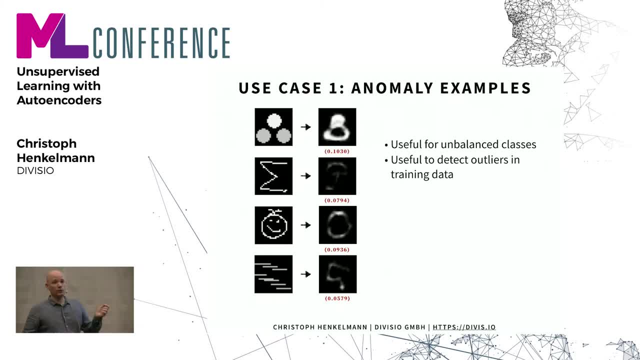 Of telling if something is wrong. You can use an autoencoder, Because you don't need a negative To detect an outlier. You don't need an example Of what is wrong To tell if something is wrong. It is also useful. 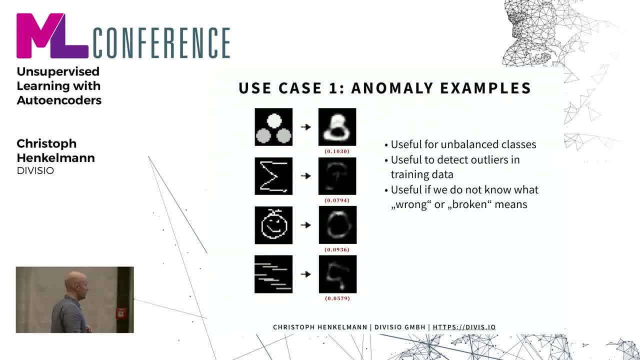 If we don't know What broken means. I mean Sometimes We want a case Where we say, If something unexpected happens, Please tell me. But how do we teach A supervised system What unexpected means? Unexpected By definition? 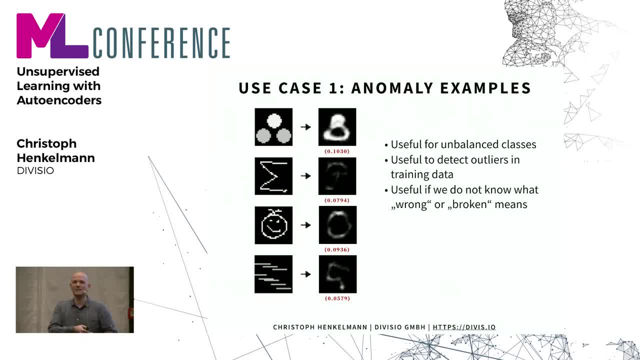 Is something we don't know. So this is why Autoencoders Can be used To detect An outlier, Because You don't need An outlier To detect An outlier. So this is why Autoencoders 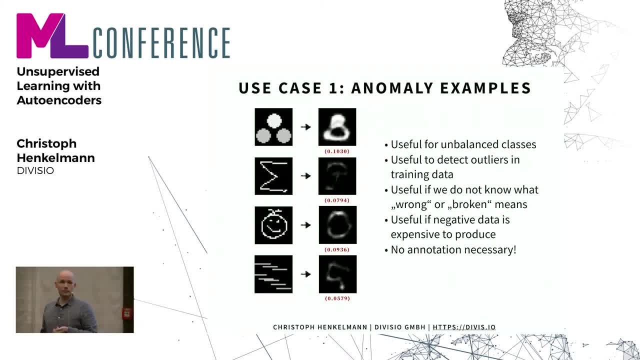 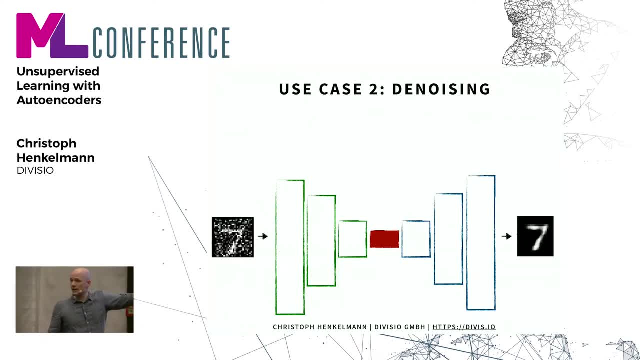 Are very useful For anomaly detection And especially Useful Also If the negative Labels Are very expensive To produce. Yeah, Let's quickly Jump to the next Idea. So We take the same idea We just had. 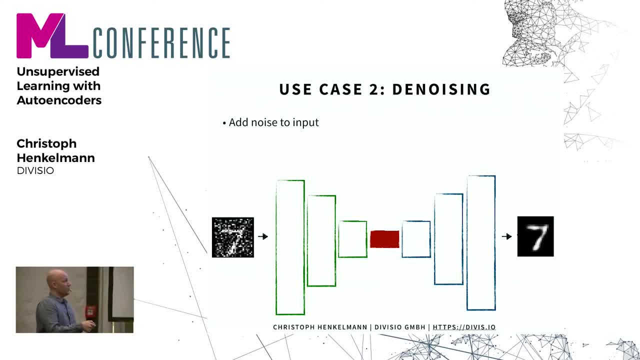 Input, Output. But this time We don't use The original input, We add noise To the input. Okay, And then Output. It's a variation. Now, Input And output Aren't exactly The same. 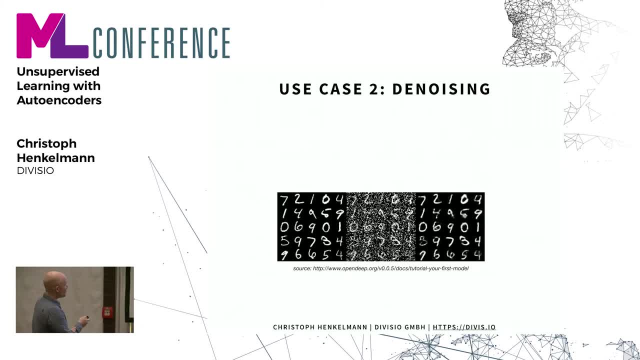 But they are Kind of The same And I didn't have time To reproduce This, But I trust It will work. Here's An example Where We feed MNIST. This is The thing. 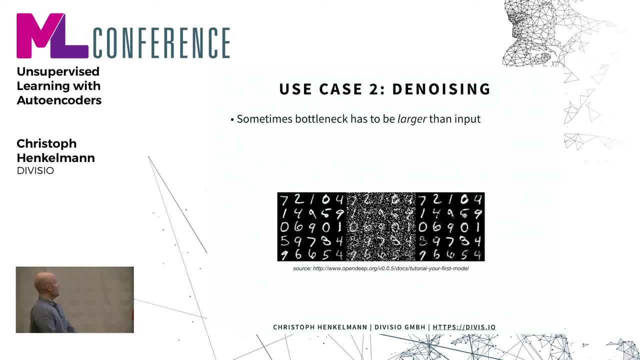 That The autoencoder Actually Sees. You see, There's A lot Of Noise In This Case. Actually Has To Be Larger. Many Denoising Autoencoders Have. 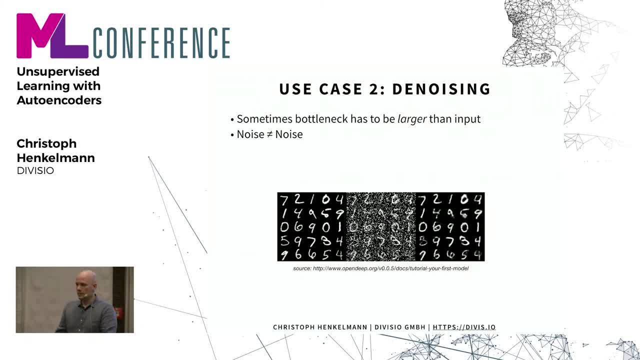 The Same Structure: A Small Bottleneck, But Sometimes The Bottleneck Even Has To Be Larger. It Looks Like Salt And Pepper. That's Why It's. 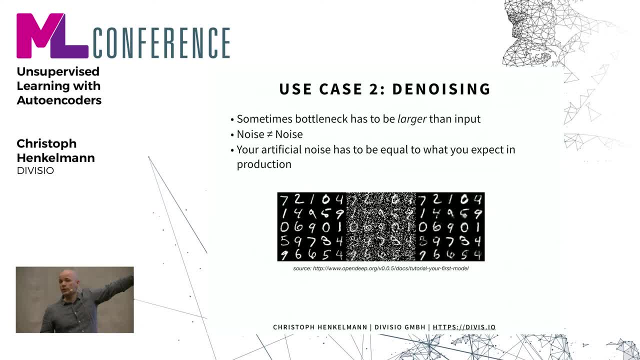 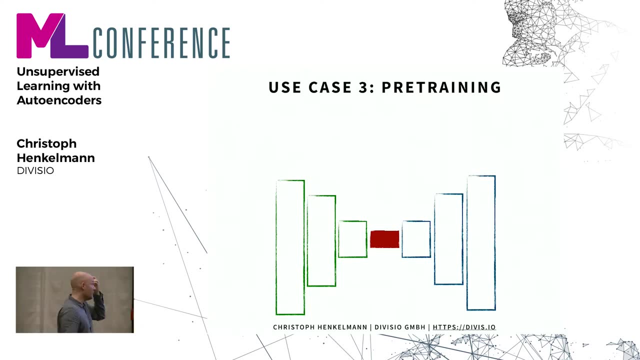 Called Salt And Pepper Noise. But If In Your Actual Application You Have A Different Kind Of Noise, They Have A Very Long Life To You. 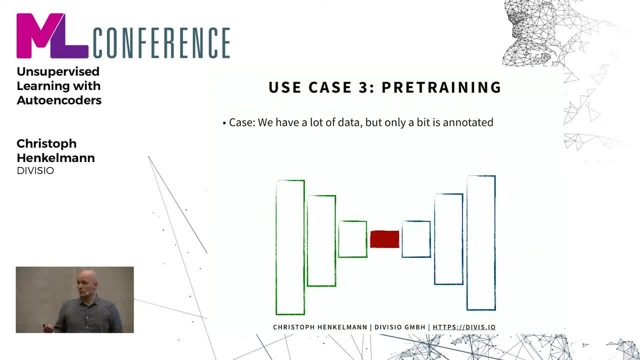 And To The Structure And The Length Of The Structure. But They Have A Long Life, But They Have A Time To, To a thousand images. okay, 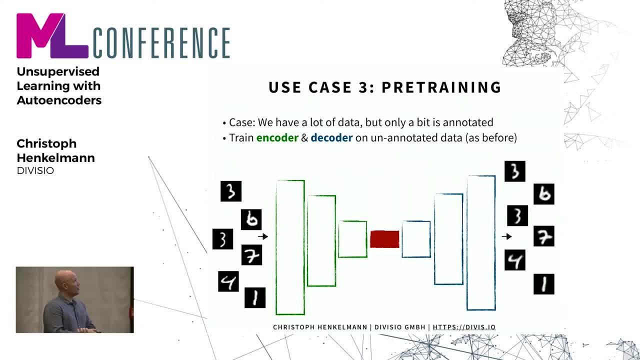 And what you do now is you train your auto-encoder, like we did before: Send in the unlabeled data, let it reconstruct the data. No difference to the first auto-encoder, right, And now comes the trick: You have this trained auto-encoder. 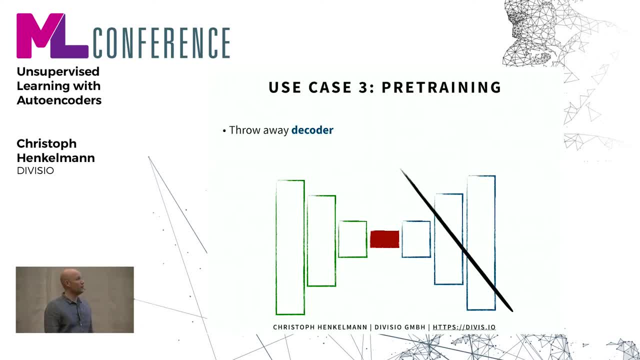 We have our trained auto-encoder, as before, And what you do now is you throw away the decoder, You break your net, you cut it in half and you throw away the blue part. It leaves you with this network. This is just the encoder and the bottleneck. 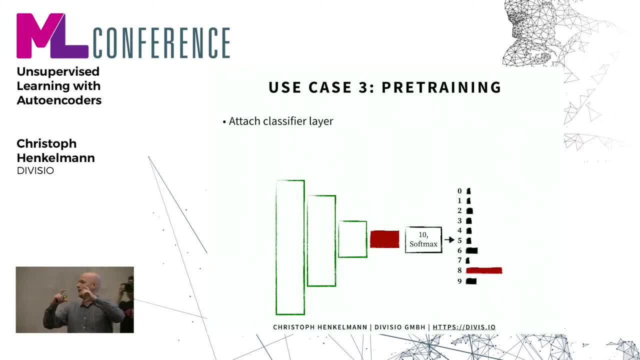 And what you do now is you glue on a new layer to your auto-encoder, a normal classifier layer, And what we do now is we take this network and do normal supervised learning, like with any other classifier that you are used to. And now comes something interesting. 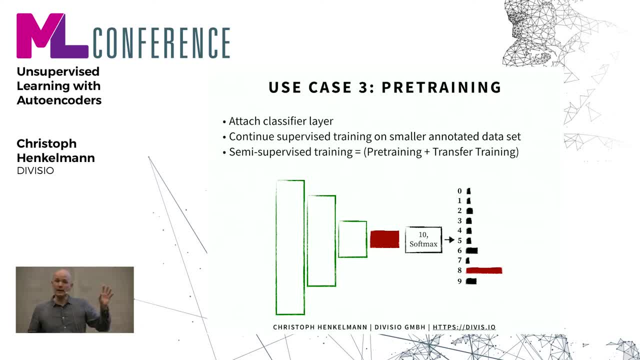 This is, by the way, this is sometimes called semi-supervised learning, because the first part of the learning is unsupervised and the second part of the learning is supervised. The first part is called pre-training and this part where we reattach. 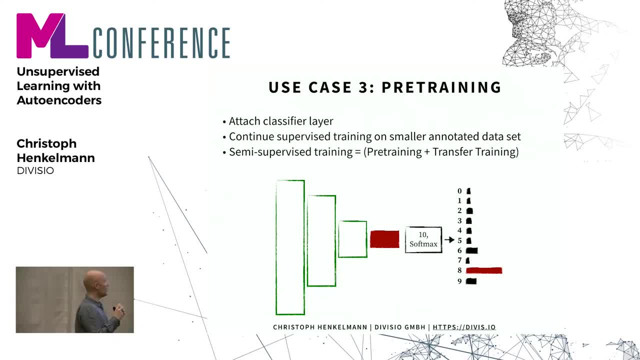 a normal, supervised part of a network is called transfer training, because we transfer our knowledge from the first part of the training in the second part of the training. Oh yeah, Just a quick. why should this work? Yeah, this is maybe what I should talk about. 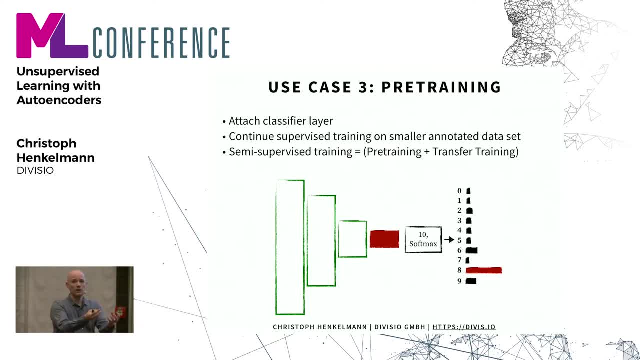 The reason why this works is that this part has learned to extract a lot of information from the original input, And what we have here is a very low-dimensional representation of our input If we have less dimension and already pre-processed and information-extracted input. 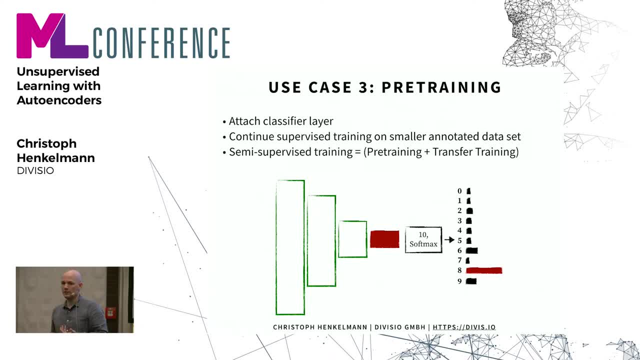 we need much less labels than we would need if we take the raw data, And the cool thing in practice is that this actually works, So you can reduce the number of annotated data that you need if you do proper pre-training. The drawback is you have to perform. 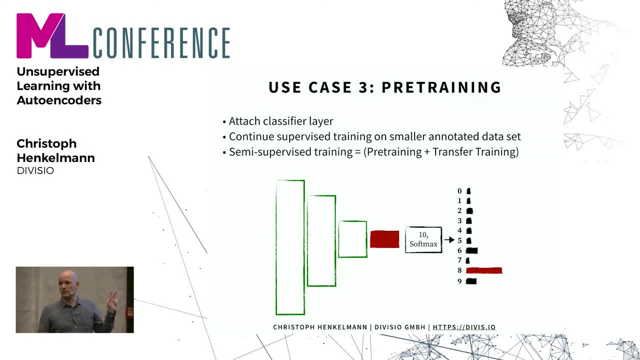 two times of training, and this is harder. So this is. it depends. If you have a lot of annotated data, just use the normal supervised version, But if you don't have a lot of data, then this can actually save the day. 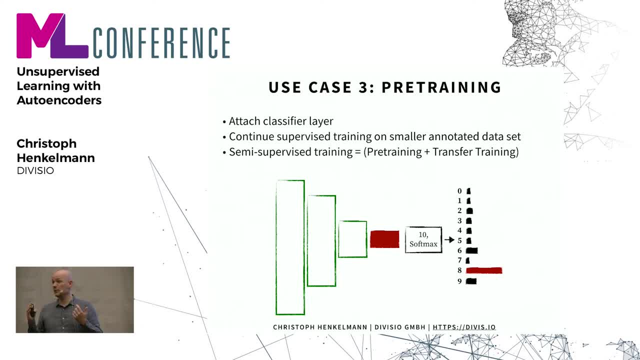 because you can save about one magnitude of data at least, sometimes more. Yeah, well, the reason is that this thing already knows how MNIST images look, so it doesn't have to be trained on doing this, And this one is just a very simple. 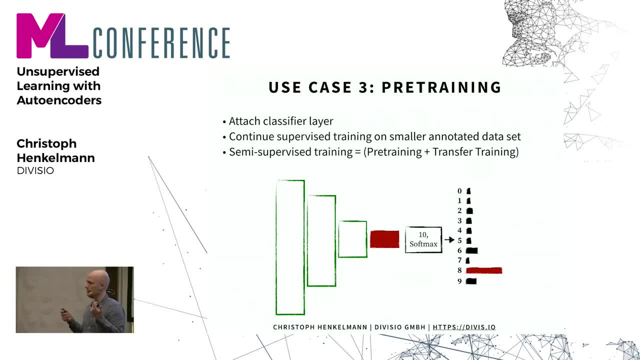 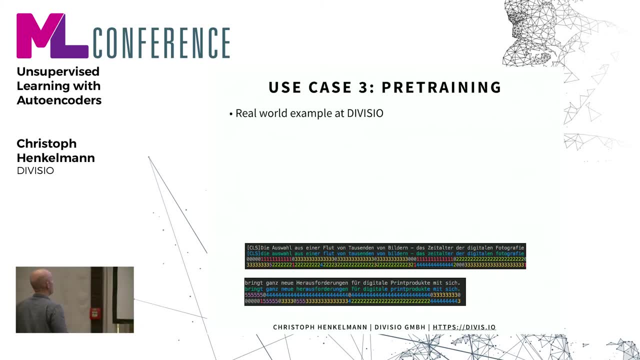 linear classifier. In many cases, the last layer is just a linear classifier, nothing more. Okay, We have an example of that in our company. This is why I'm so happy about this. This is a project We are building, an in-house product. 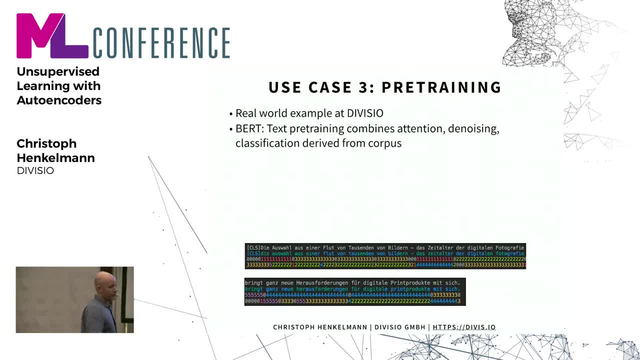 at Divizio And maybe some of you have heard of an algorithm called BERT. It was in some of the other talks, I think in the talk about chatbots. we have heard about BERT already. It's one of the coolest NLP algorithms. 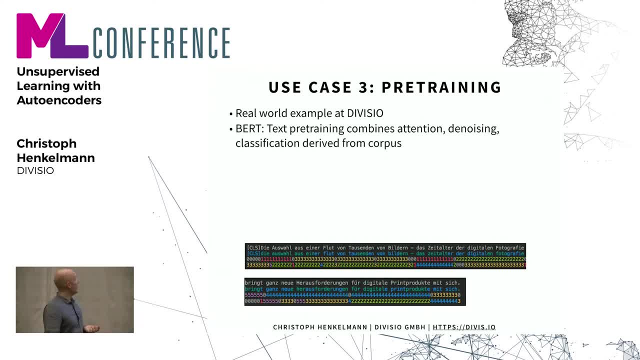 in the last years. It came out in September last year And normally if you talk about BERT you wouldn't say BERT, like in Sesame Street, by the way. Yeah, BERT, as in Ernie and Elmo. 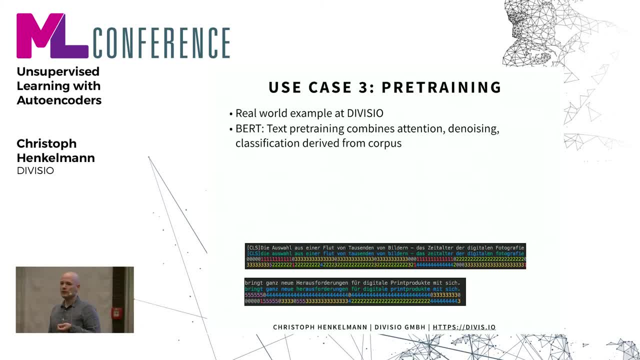 You don't think of BERT immediately as an autoencoder, but technically it is a denoising autoencoder, actually with a very, very much more complex structure than I've shown you, But in essence it's a denoising autoencoder. 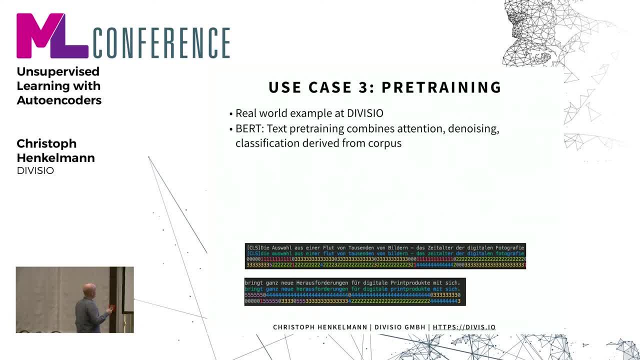 And it does pre-training on Wikipedia. So what you can do is you just take the whole of Wikipedia. You don't even look at it, You don't annotate it, You do nothing with it. You just take the Wikipedia text and run it. 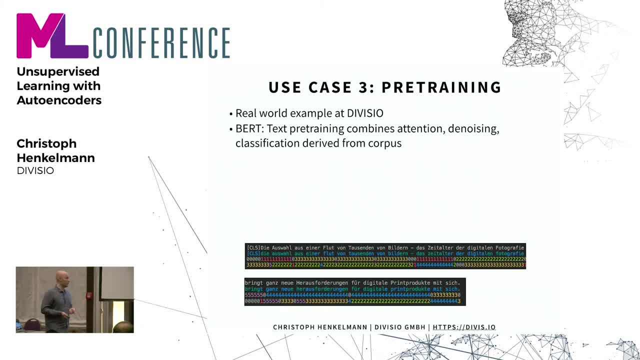 through BERT for days. Yeah, BERT training- depending on how you do it, takes four to 16 days. And then why did we do this? Because our product is an NLP product and we needed our own part of SpeechTagger. 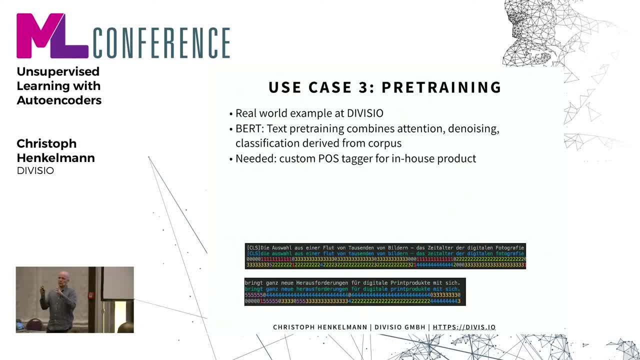 Part of SpeechTagger takes a sentence and attaches meaning to certain parts. A part of SpeechTagger could, for example, say: this is an adjective, this is a noun. More complex part of SpeechTagger perform, for example. this is the subject. 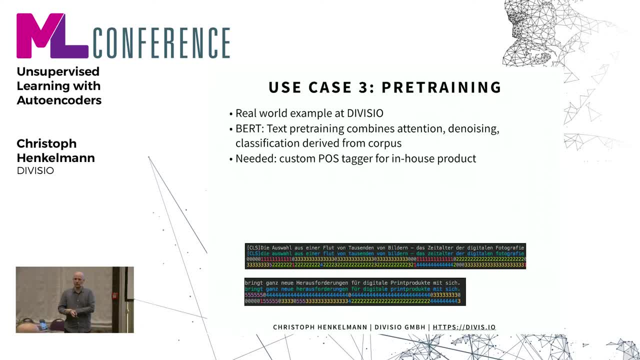 of the sentence. this is the object of the sentence. That is called part of SpeechTagger And we needed- for reasons I don't want to go into, we needed- a custom part of SpeechTagger that tagged in a way that no other part. 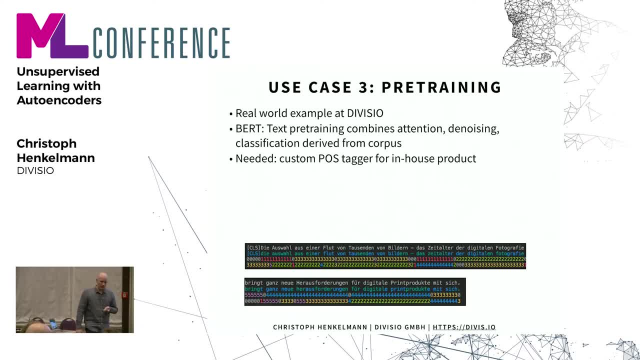 of SpeechTaggers do, So we needed to build our own one, And normally a part of SpeechTagger needs at least 10,000 examples. Better more: 100,000, 200,000 sentences. Yeah, Pre-training. 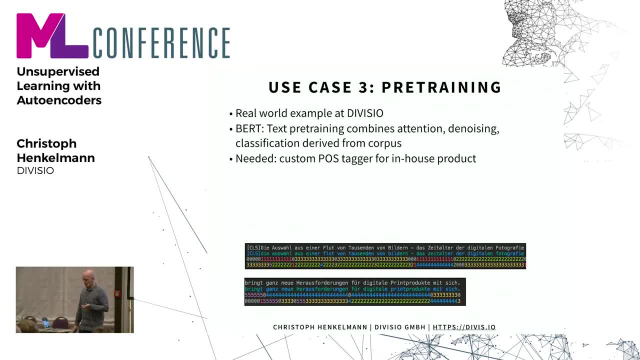 Let's do this later. So the problem is, we are not a big company like Google, So we can just say: well, let's hire 50, 50 German students and let them annotate sentences for four months. We don't have the money. 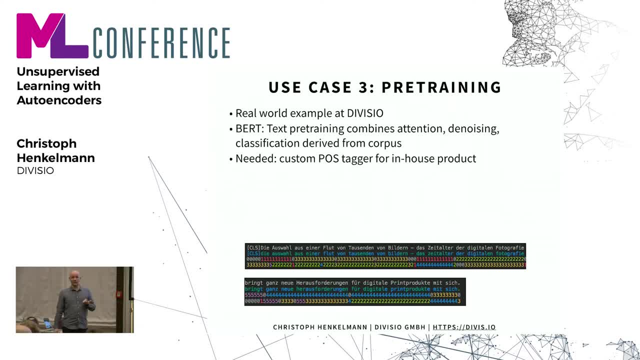 and the time, So we needed to do something faster. So the data was annotated by me and a colleague. Took us a week And we produced 1,000 sentences And we combined this with BERT And the first test we did run. 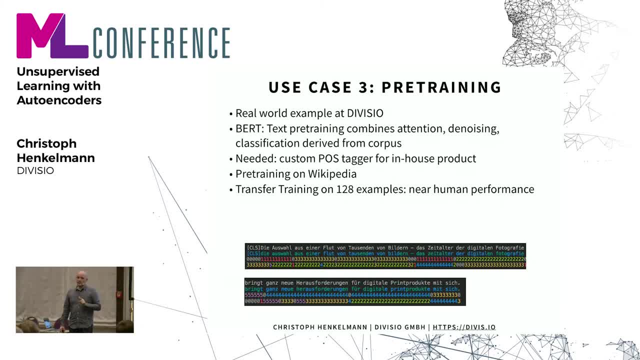 after two days of tagging, we only had 128 sentences, Because sometimes this shows how expensive annotation can become. Sometimes we needed to discuss a sentence. It's a colleague of mine. she and I. we discussed a sentence for five minutes to find out. 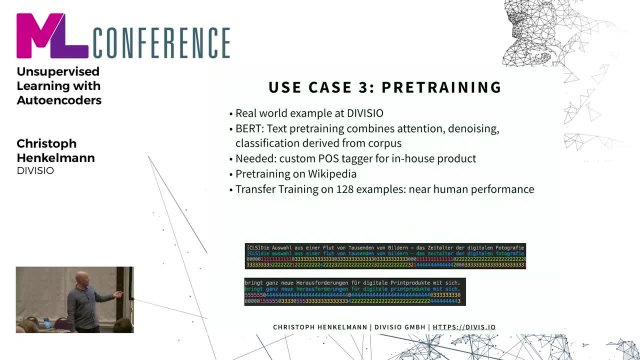 what the proper grammar is, because it's a really hard task And we trained, we did transfer training with BERT on 128 examples and was already near human, So it was already about as good as we were, And after 1,000,. 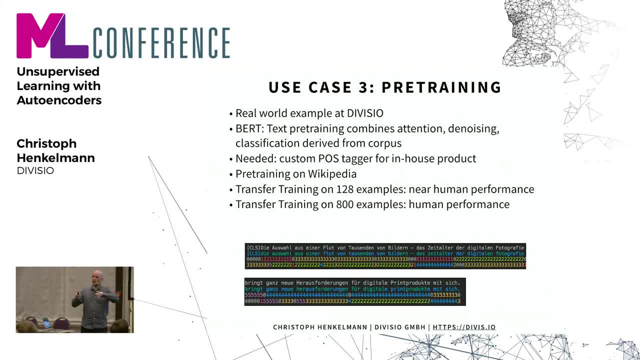 actually the training set was 1,000 examples. we split it up into 800 training and 200 validation, And after 800 examples the performance of the model was the same as our own performance. So instead of needing 100,000 sentences, 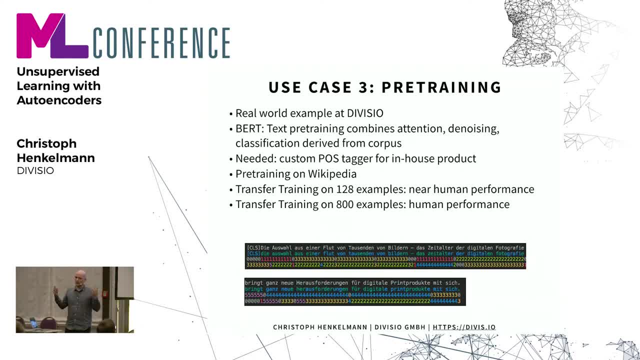 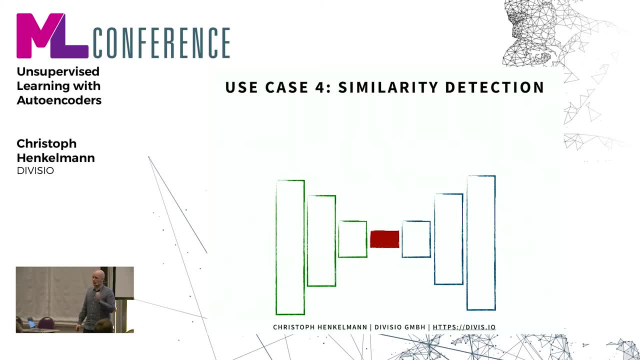 we could do it in 1,000. So for a company like us, that is like it's gold. You hit gold, Yeah. So this transfer training thing is a great way if you have a lot of data but not much of it. 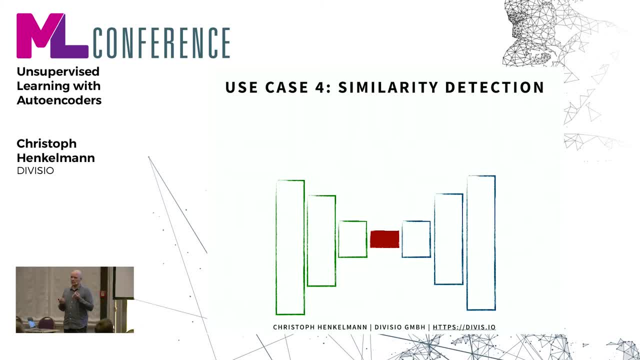 is annotated or it's very expensive to annotate. Sometimes it's cheaper to work for a month on a custom autoencoder than to pay- I don't know- 100 people for months to annotate two or three orders more. It's more of a magnitude. 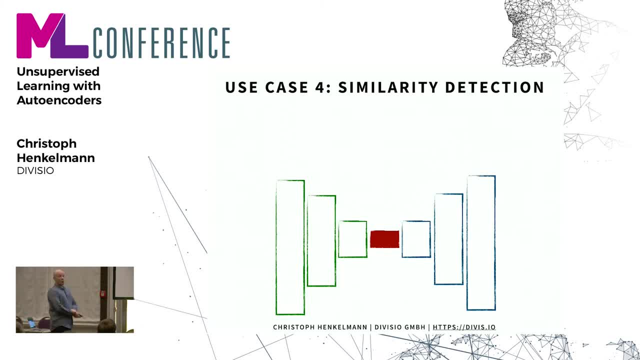 of data. Okay. So what else can you do? These things are the gift that keeps on giving. You can do even more with them: Similarity detection. So you do the same thing as with the pre-training right: We train normally. 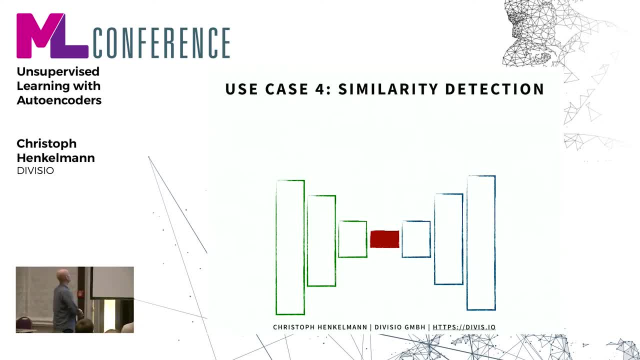 like we train our autoencoders, Same thing. So again we throw away the autoencoder and now we don't attach anything. This is nice, because this is much simpler than the transfer training. What we do is we feed it, our data, into the network. 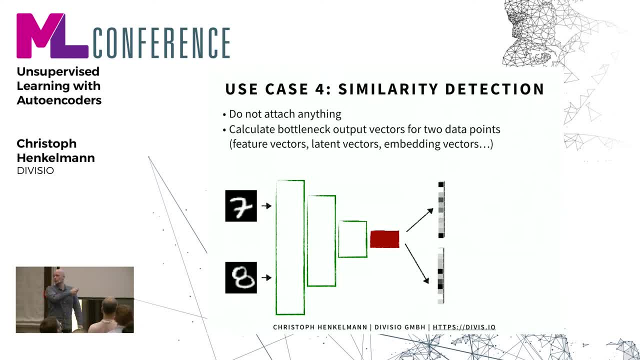 and what we get here are our representations that are produced by the bottleneck. It's just, it's a representation of the data with much less dimensions. These representations have many names. Sometimes they are called feature vectors, latent vectors, embedding vectors. Depends on. 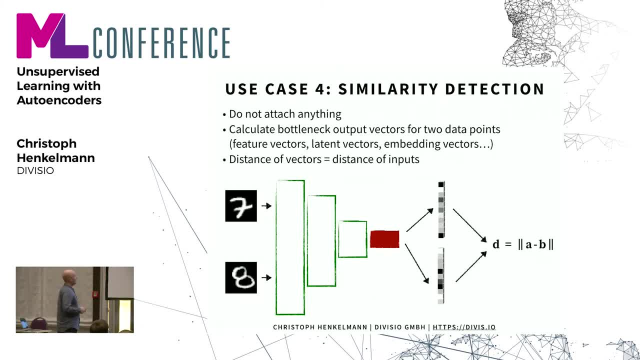 the context that those words are used. And now we have two vectors and this is the only bit of math in the whole slides, I promise You just take the distance of two vectors. There are many ways to calculate the distance, depending on what use case you have. 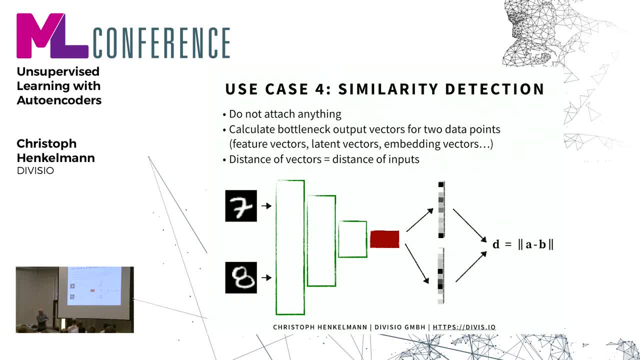 Some work better than others, But what you can tell is here how similar these vectors are, simply defined by the distance of the vectors, And what you have built now is a neural network that can tell you if two inputs are approximately the same. It's something. 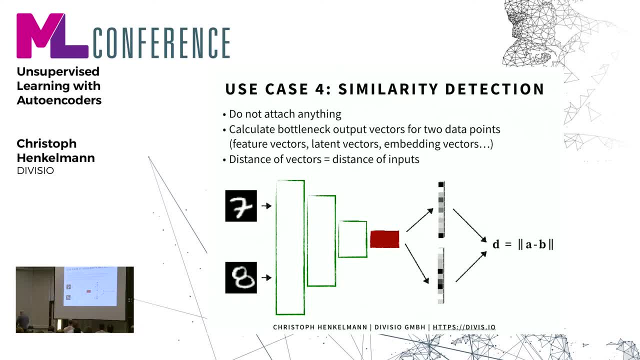 we humans are really, really good at. I could show you these two bottles here. Just grab anything and you'd say, yeah, they're about the same. They have a little difference, different cap, but they are basically the same model. If you do this, 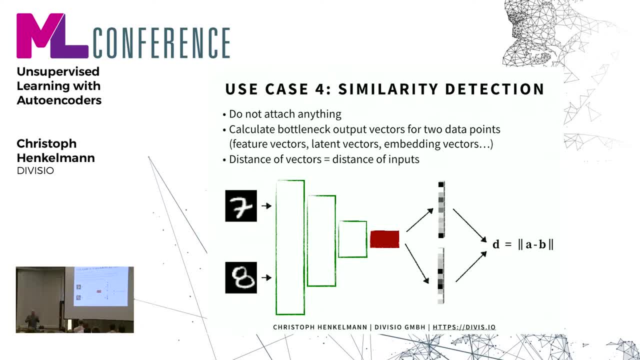 just with a JPEG. if you just move an image by one pixel, a normal pixel comparison completely breaks down And what you get with this is a fuzzy comparison of inputs. Depending on what you work in, it's a very useful thing, For example. 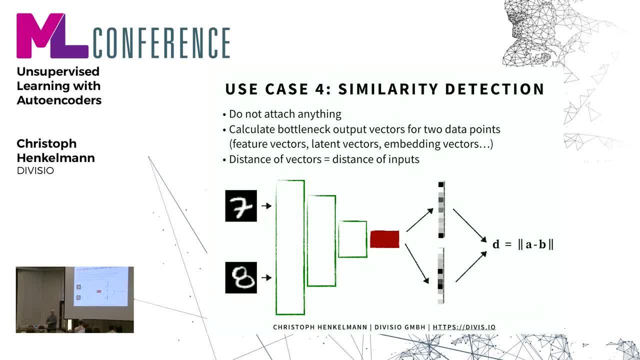 if you build chatbots and you want to find out if your intent is matched or not, you can do something like this on your. This is actually, by the way, how those chatbot intent matchers kind of work. They use embedding vectors. 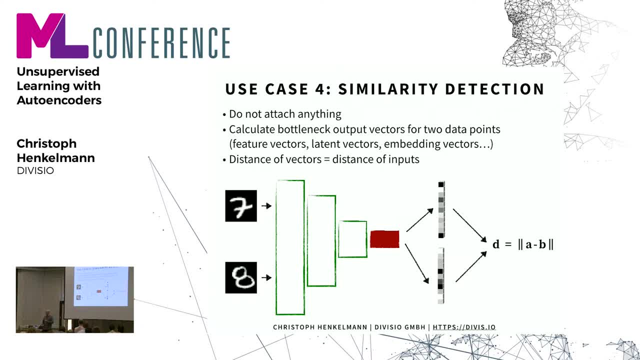 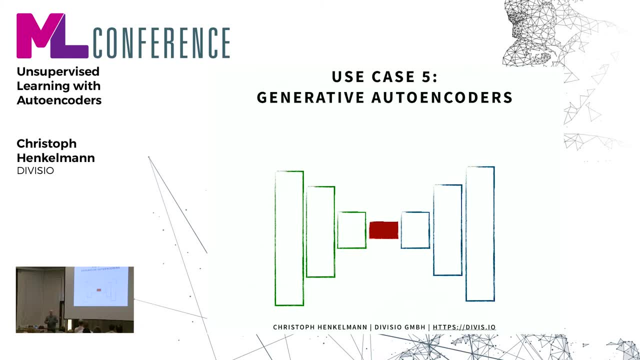 and calculate distances. There's some Maybe, maybe not Kind of, And oh yeah, that was the fourth use case. We can do something else. We still take our normal autoencoder. We do the same training as usual, but this time. 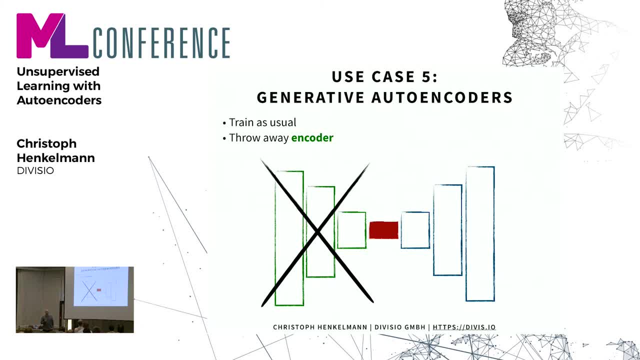 we throw away the encoder. So it's funny about autoencoders: If you throw stuff away, it gets better. So we have this. So how the hell can this be useful? Well, if we put noise in here. this layer has learned. 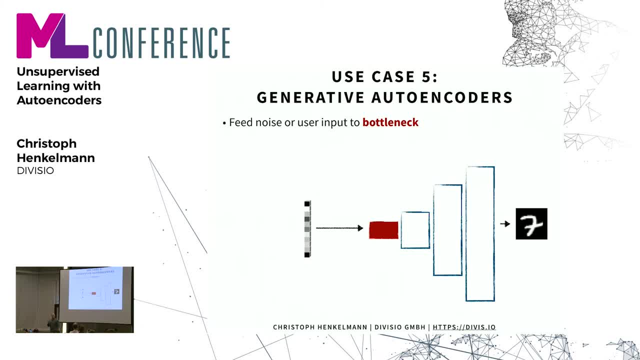 to reproduce input based on latent vectors. So if we feed it a new latent vector, we can generate new data. So if we feed it the right vector, suddenly this will turn into a seven And with that you can yeah. 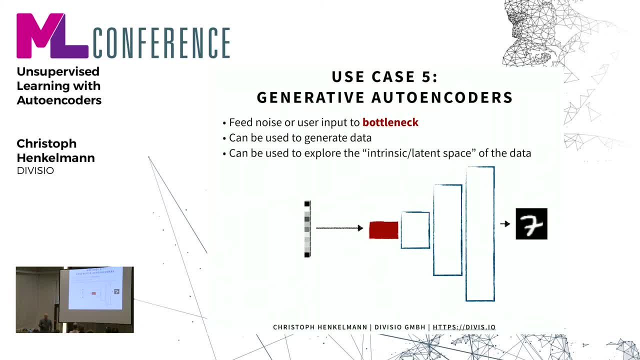 as I said, you can generate all kinds of data, but there's something that is more useful about this: You can explore the so-called latent space. Okay, this sounds very science fiction-y, but it isn't. You can use this as a way. 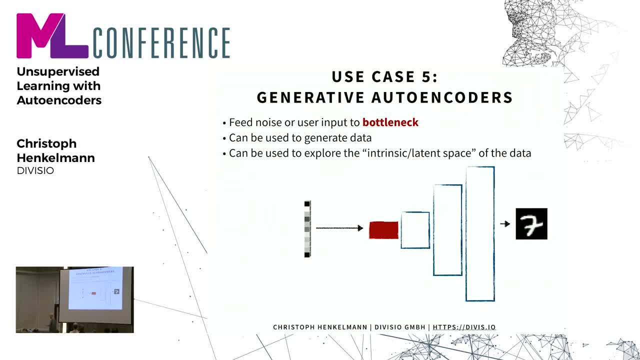 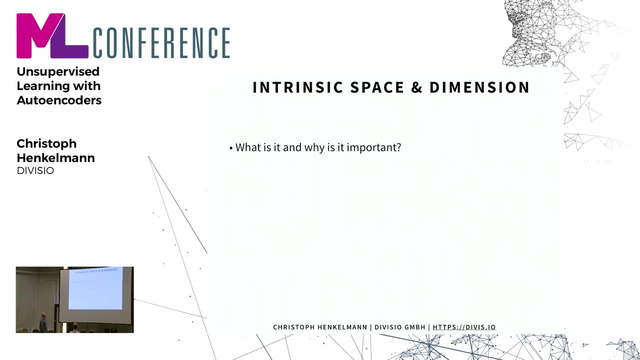 to actually explore the data you're working with. Let me let me illustrate this a bit more. We have the terms intrinsic space and dimension. This is much more complicated, much less complicated than you might think. So what is this and why is it important? 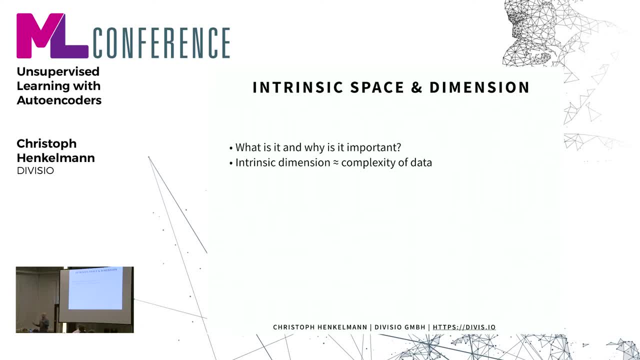 The so-called intrinsic dimension is the complexity of your data. Okay, Our MNIST data set technically has a dimension of 786, I think, for every pixel. Every pixel is a dimension, But in reality it's much simpler. We only have 10 digits. 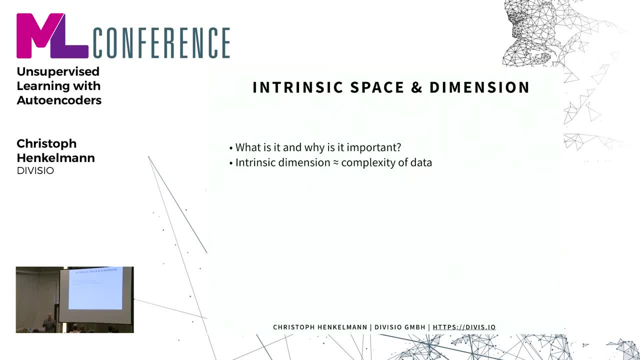 and some of the digits come in various varieties, So we have maybe two dozen dimensions that actually specify how a number looks Okay, And so the MNIST problem is actually much less complex than the data would look, So it's not as complex as a 700-dimensional space. 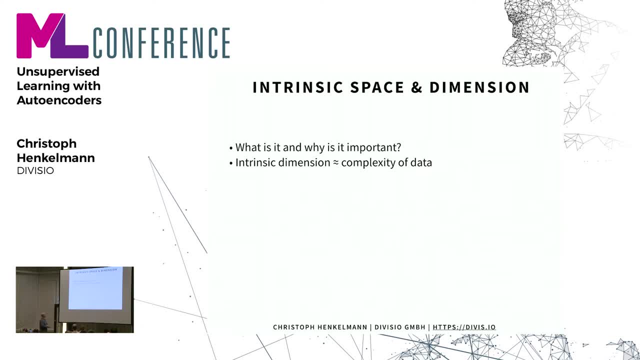 It's just as complex as a- well, maybe 20-dimensional space. And the thing is, if we know how complex our problem really is, this will help us design our system, Because if a system is too complex, too big, too large, 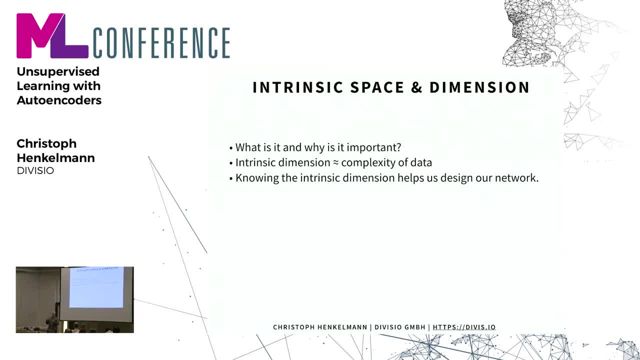 if the model is too large it will tend to overfit, But if it's too small it will not do the task. Normally we try this bit by bit, We try this variation and then at some point we luckily arrive at a model that's kind of right. 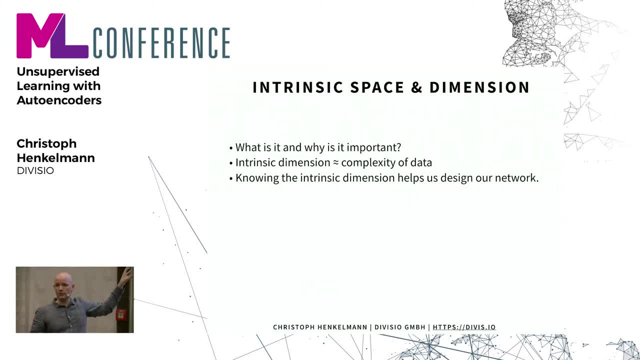 But if you explore, if you know what your intrinsic dimension is, if you have another image data- say, you have a similar image like MNIST, but they contain much more complex images and you know the dimension is 100, okay, then you will. 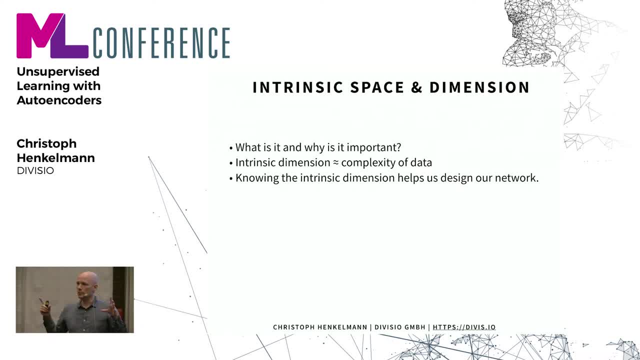 quickly say: well, we can't use the MNIST network for this, We need a bigger, more complex network. It will save you time. And the perfect autoencoder is, of course, the one where the bottleneck has exactly the size of the intrinsic space. 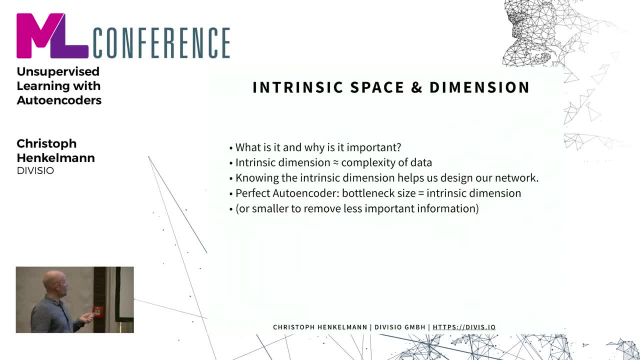 That would be the perfect autoencoder. The problem is: or smaller? yeah, if we want to remove information, if we want to keep the most important information, we want to make the bottleneck small, even smaller than our intrinsic data. So the problem: 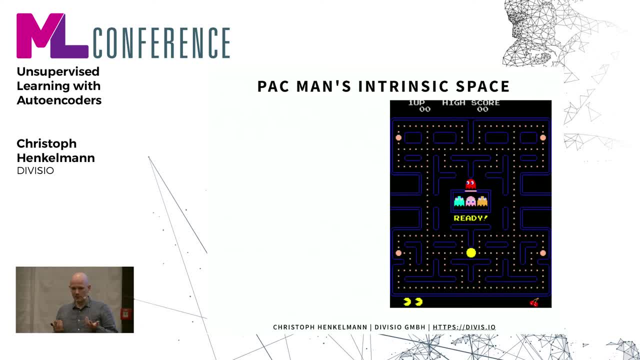 is high-dimensional intrinsic spaces. It's such an abstract concept. There are images that mathematicians do of high-dimensional shapes. They look nice, but they don't tell you anything. So I have a different example. Let's look at the game of Pac-Man. 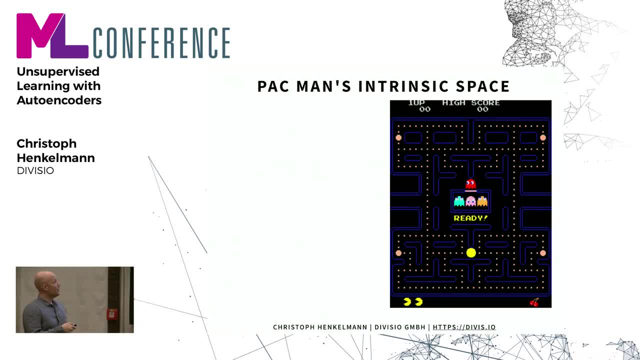 I guess everybody is familiar with that one. And let's look at the intrinsic space of a Pac-Man Pac-Man screen. The input is much larger than our MNIST, It's something like 50,000 pixels. It's an old arcade machine. 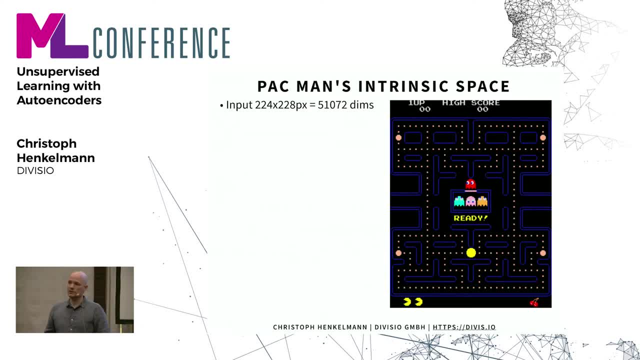 so luckily it's not high-res or anything, but still, 50,000 dimensions is not little. But what is the information on this screen? Let's look at the information We have: the number of lives down here, That's one dimension. 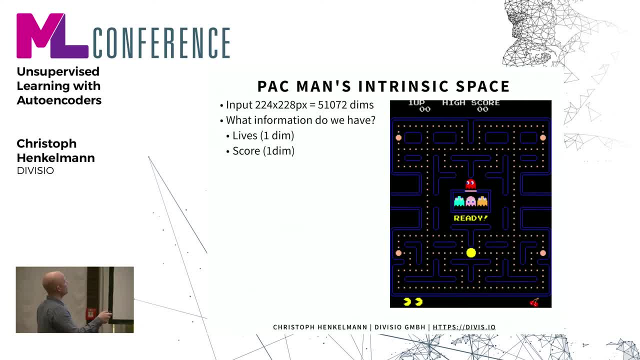 That's one number. We have the score. I think it's that one. We have the high score, We have the level we are currently at. Now you might say, well, what we actually have is the positions of the walls. 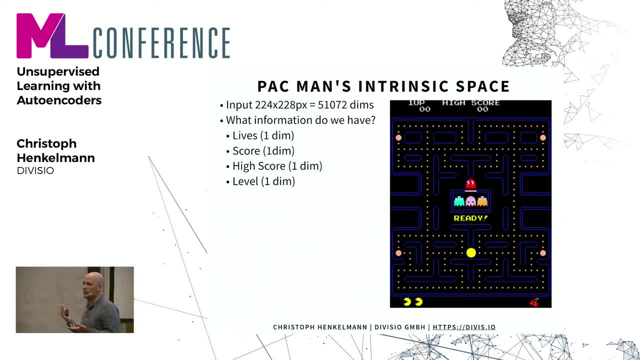 but Pac-Man is a finite game. There's not an infinite number of levels, So there are just, I think, 255 levels, And the levels never change. So if I know which level I am in, I know where the walls are. 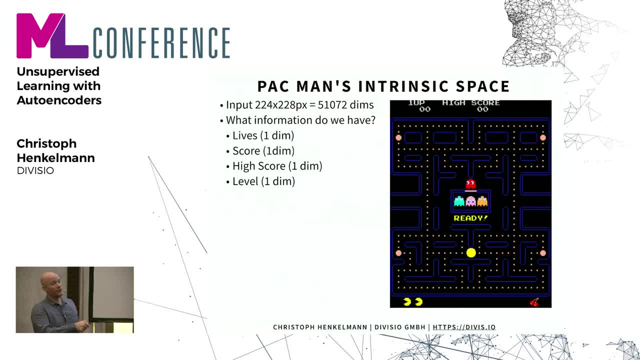 I know how the maze looks. So actually the maze itself is just one dimension. We just need one dimension to encode which level we are in And a good auto-encoder will decode just from the number the shape of the maze, Because the yeah. 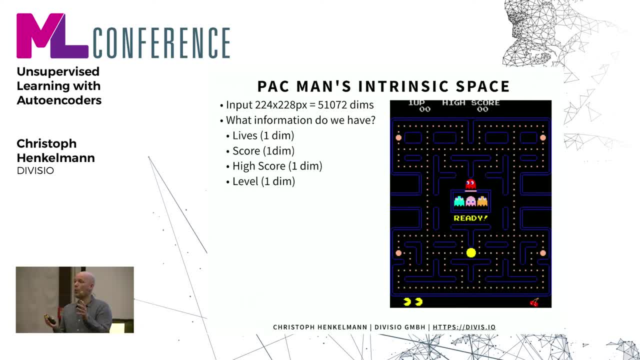 It looked like you wanted to ask it. The decoder will store the information how the different mazes look, So all you need is one number to decode the maze. You have the pill state. I did a quick count. I think there are no more. 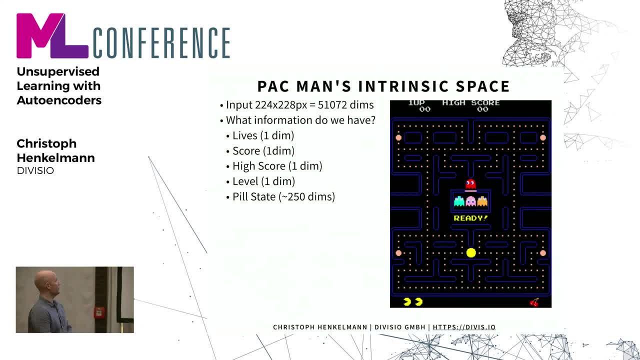 than 250 pills. I just yeah, let's say roughly 250, depending on the maze you're in. We have our ghost positions. It's XY, four ghosts, XY positions, so eight dimensions. We have the Pac-Man position. 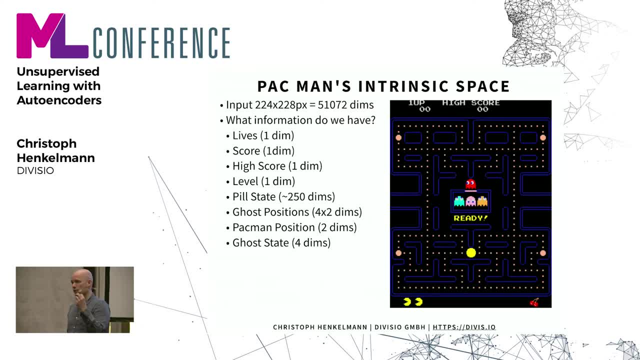 We have the ghost state. Ghosts can be aggressive, They can chase you or they can be eaten. So they have. each of them has a state And Pac-Man has a state. He can be alive, He can. maybe he can. 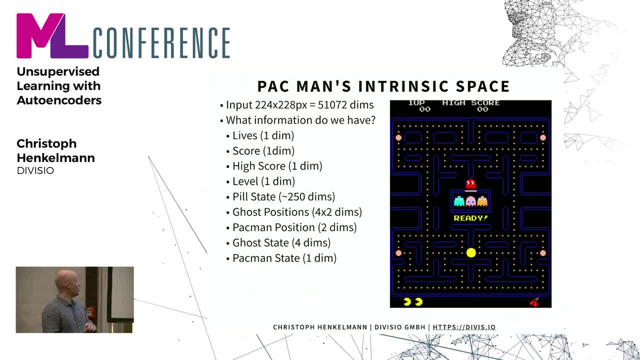 he's before the game starts. He has a different state, But you can encode it in one dimension And you have the game state itself Running ready. start screen, high score screen. And I probably forgot something, because it's a long time. 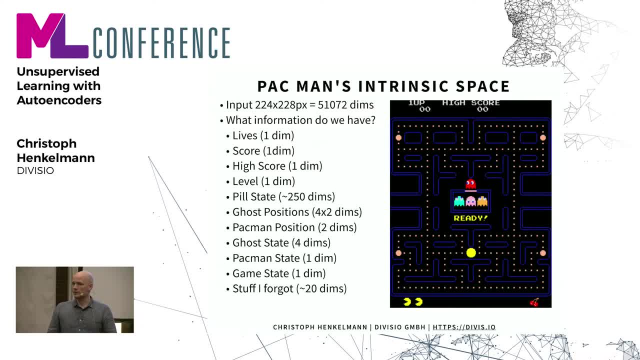 since I played Pac-Man. So just say, 20 or so more dimensions for stuff I didn't think of. If you sum this all up, you actually have less than 500 dimensions. So you know the intrinsic space of the Pac-Man game. 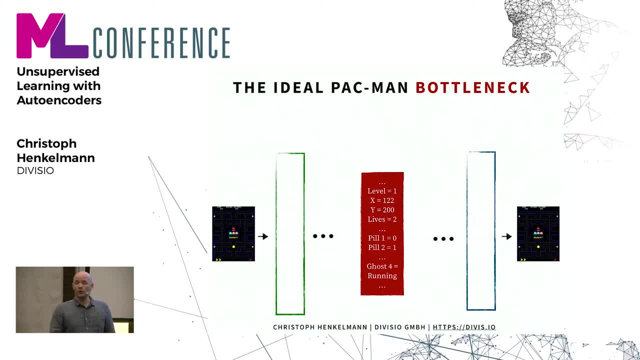 is 500 and not 50,000.. That's actually only 1%. So a perfect Pac-Man bottleneck would look something like this: It would have- it's a bit larger so I can add the text, but it would only have 500 neurons. 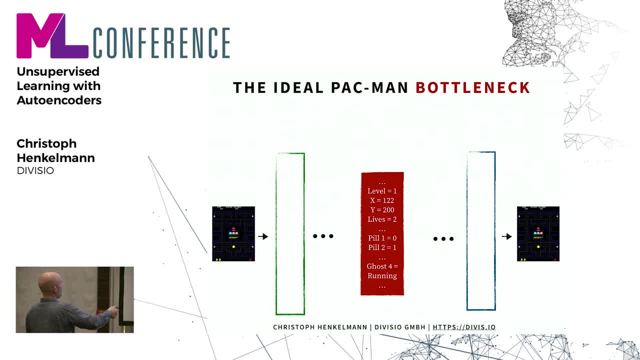 give or take And it would take as input an image. Then it would encode the image And the cool thing is, if we have a perfect Pac-Man auto-encoder, we could actually read the game state from the neurons And then we feed this. 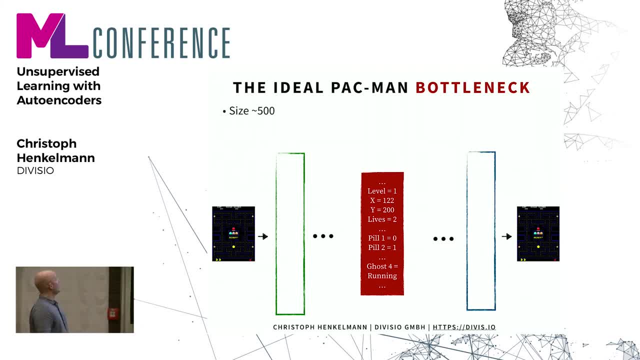 into the decoder and we should get the original image back, Would have a size of 500.. Yep, that's what I said, And the important thing is that each neuron would actually mean something That is very useful. We have normally. we have these black box. 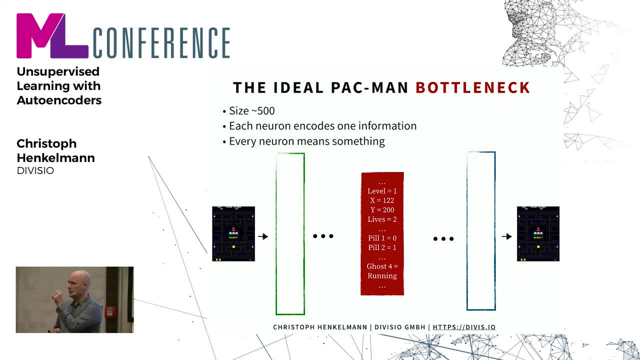 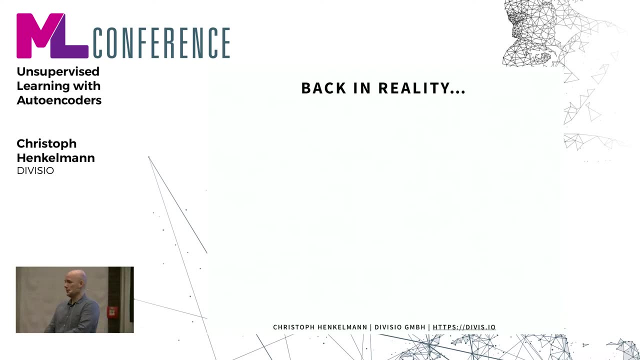 neural networks. We don't know what those neurons do, And here in the ideal auto-encoder, each of the bottleneck neurons would actually tell us information that is useful. Okay, So back in reality. This is easy. I mean, what is those? 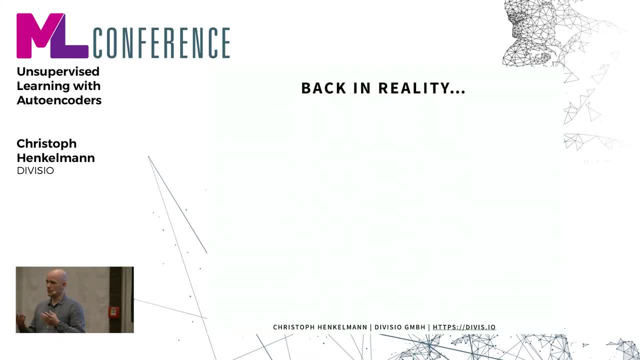 you know those game competitions that people do, where the reinforcement bots learn automatically. So what's so hard about this? right, We just teach an auto-encoder and those, what's the shooter or that game they were playing? We just encode. 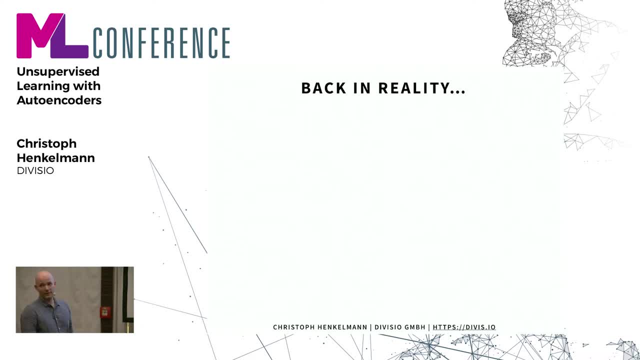 the game state and we can win Easy. Well, sadly, it's not that easy. What normally happens is that our dimensions are spread across neurons. Okay, When you have this example, this virtual example I just showed you, one neuron means 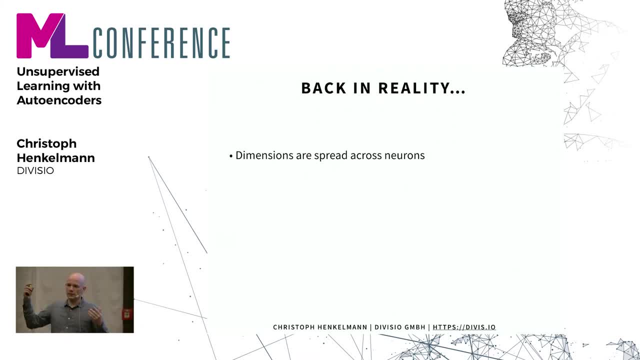 Pac-Man's lives. But this is like having a line in a vector space, and this line can have a different shape. So we have no guarantee that actually each axis our neurons represent actually encodes only one piece of information. What normally happens is that the dimensions 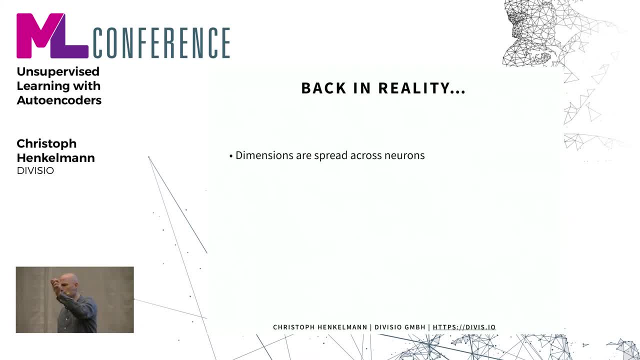 are smeared. So the first neuron encodes a bit of the Pac-Man's lives. The second to last neuron encodes some of Pac-Man's lives. So it will be quite a mess And generally the auto-encoder will use every neuron it can. 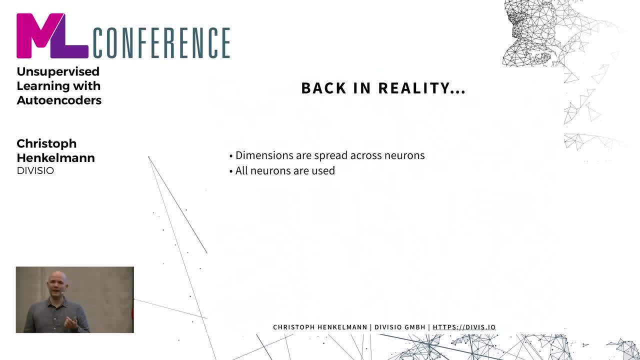 It's very hard to tell which neurons are useless. Mostly they aren't. A normal auto-encoder will try and use everything it can, And what we actually have to do in practice is we start with one auto-encoder that kind of works. 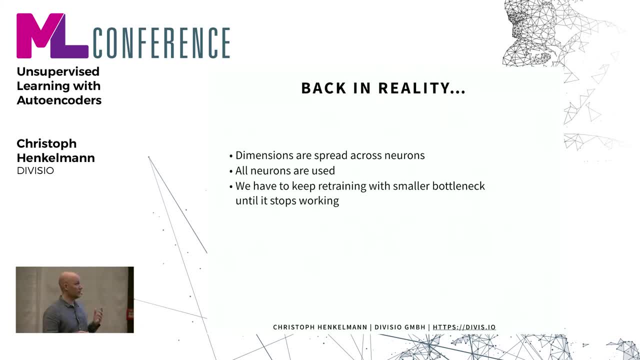 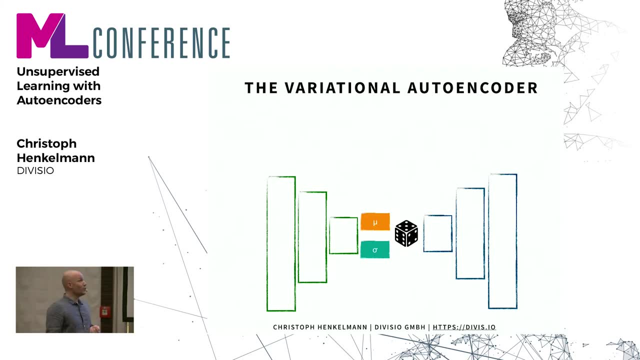 And then we reduce and reduce and reduce the complexity of the auto-encoder until we find one that stops working and we go a step back. But there's something even cooler to fix that. It's the variational auto-encoder, And I will not go into details here. 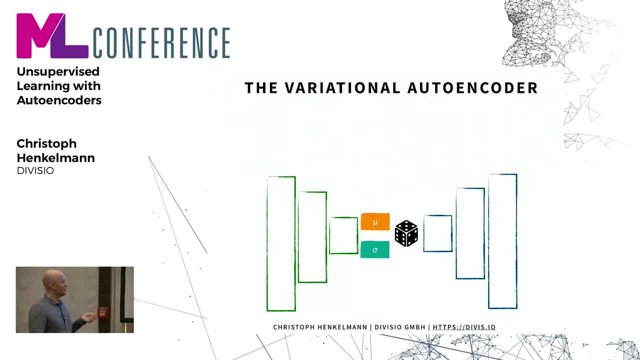 because the principle is relatively simple, But why it is the way it is is a bit hard. But the variational auto-encoder has an idea. The idea of the variational auto-encoder is to punish bad encodings, Normally with an auto-encoder. 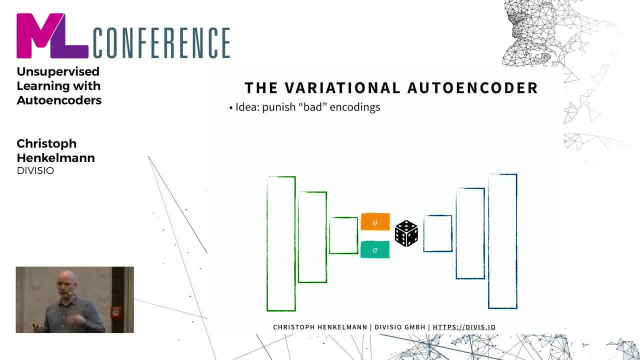 we punish bad reconstruction. This is our loss function. in the neural network We compare the input with the output, And if they are too different we have a large error. If they are actually almost the same, we have a low error. The variational auto-encoder. 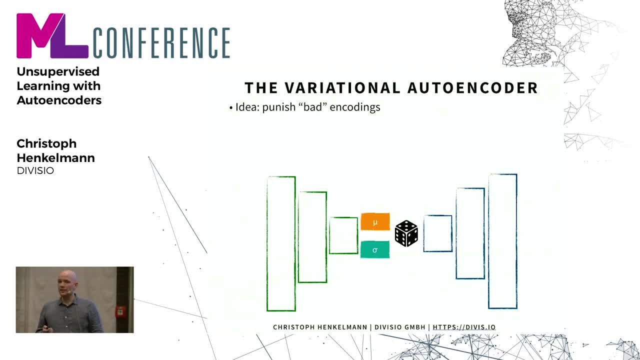 adds a second loss term to our training, And this is the quality of the bottleneck. So the idea is, if we have a good bottleneck, we have a low error. Sorry, if we have a bad bottleneck configuration, we have a high error. 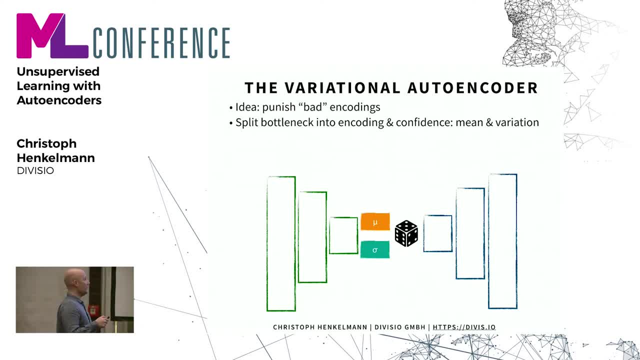 And how do they do this? What they do is they do not represent one latent vector, but what it produces is a probability for a latent vector. I will show you in a moment a bit more what this means. but we don't say neuron number five. 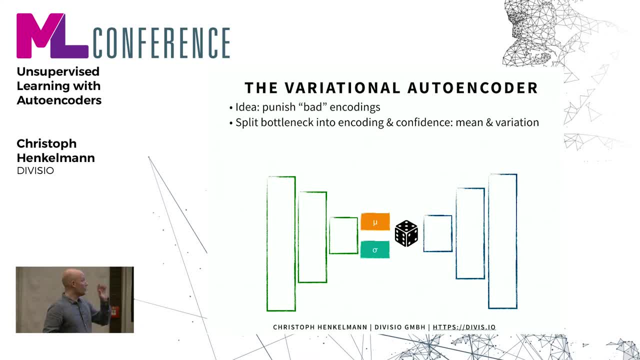 has value 0.5.. What it says is: neuron number five has an average value of 0.5.. What it says is: neuron number five has an average value of 0.5.. What it says is: neuron number five has an average value. 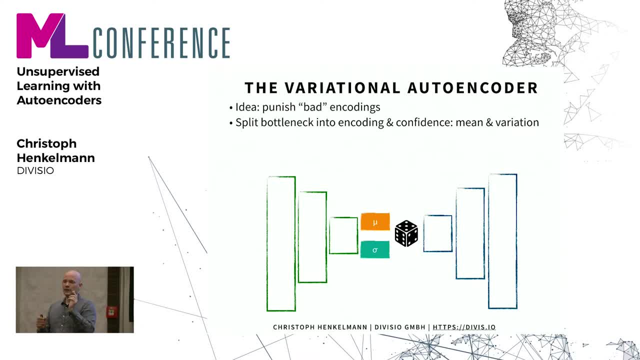 which I expected to have a value of 0.5, but I am not sure about it. So we spread. you have a variance. So the encoder part actually doesn't tell you what it thinks the latent vector is. It tells you what it thinks the later vector is. 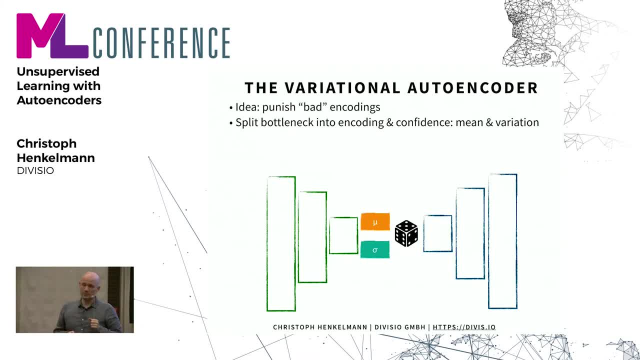 and it tells you how wrong it might be for each of the inputs And what you actually do, what the decoder does. of course the decoder has to get a vector right. It has to get an input vector. So what it actually does. 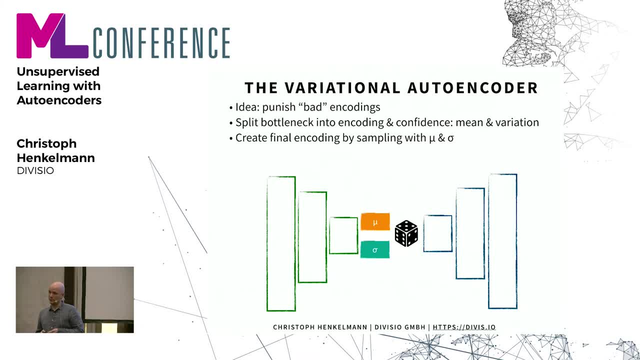 something very unusual for a neural network. there's a random number generator built in, And what it does? it samples one possible latent vectors from the distribution that is created by the encoder. The useful thing about this thing is that that way you don't get hard boundaries. 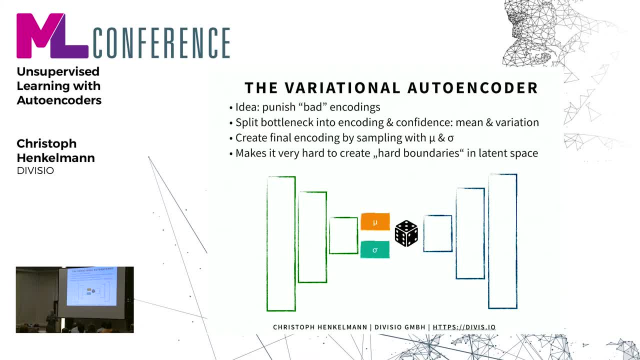 What a normal autoencoder will do. it will there might be, if you think about, let's just assume the bottleneck had size two right, So it's like. it's like a plane, And what might happen for one neuron is. 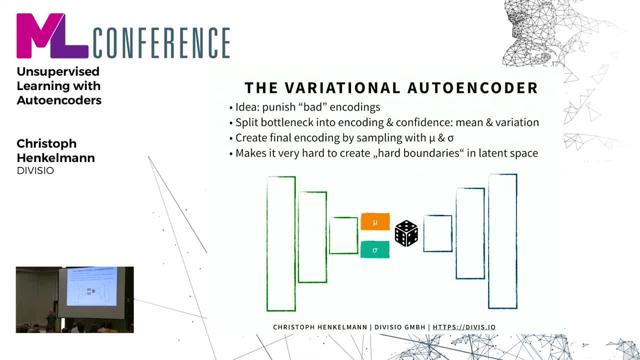 that there's a useful configuration for the neuron that is here, And suddenly if you move the value of the neuron here, it will produce totally useless output. It will produce a latent vector. that doesn't make any sense, But because here we can never be sure what the decoder will sample. 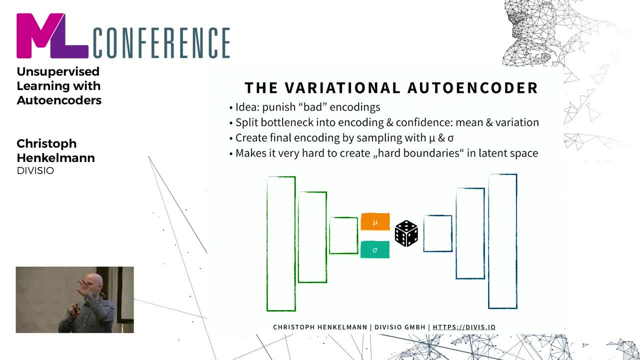 it forces the encoder to move the values of the encoded neurons So they have a nice smooth surface. So your whole latent space, the whole information you want to encode, is one smooth surface. And this makes the reconstruction much easier, because if we build a generator by just using the final part, 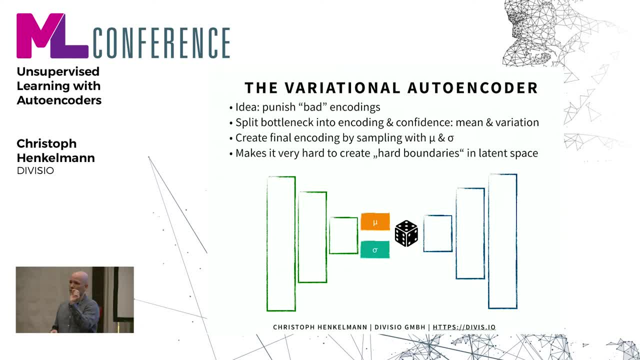 with a variational autoencoder, we can smoothly run the latent vector from one point to the next and we'll see the image change smoothly and produce useful output. I have an application that does this with MNIST. in a moment, Bear with me a bit more. 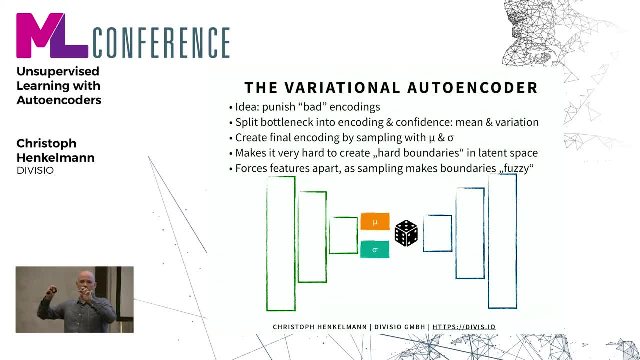 But the other thing is also it forces the features apart. because the boundaries are fuzzy, The features are forced to move apart. So I have one feature here in one neuron and another feature in another neuron And because they are sampled, those features are moved apart in the internal representation. 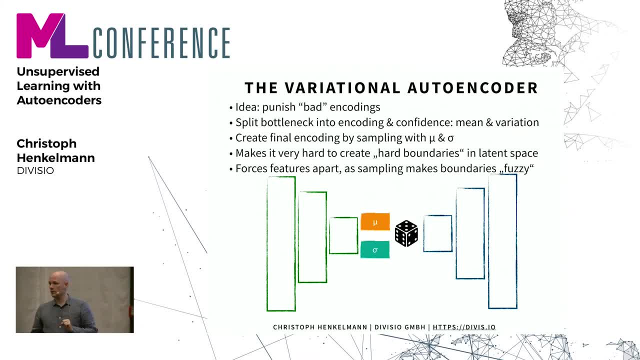 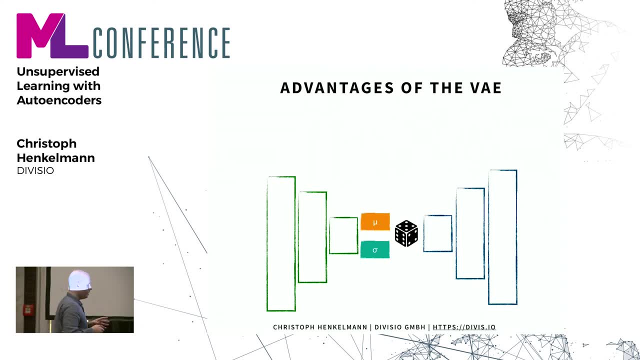 So each neuron becomes more meaningful. Just for one aspect. Variational autoencoders are. Don't worry if you don't completely grasp the concept. It took me quite a long time and many tutorials to read to completely understand how they work internally. 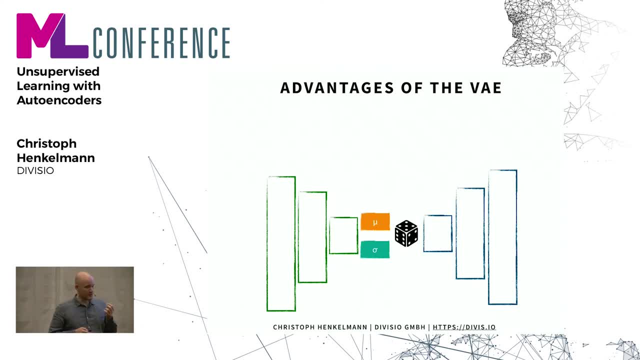 And what I suggest you do is you should remember variational autoencoders sample internally. The bottleneck is not completely deterministic And you should just remember what the advantages are. What is the output that is created? The features are more likely encoded in separate neurons. 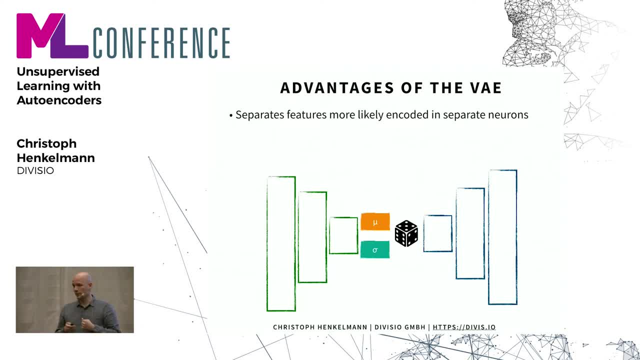 So the features are not so much smushed together into one neuron. And the cool thing is- and this is one of the nicest thing and we will actually see that it works- worked on the first attempt, which is kind of cool. 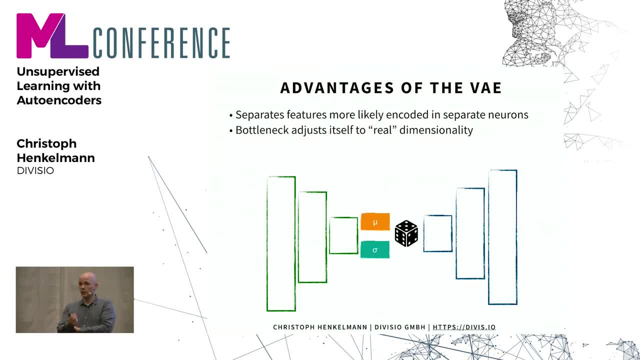 is that you only get as many neurons. only as many neurons are used as you actually need. So normally, I told you, with a normal autoencoder it will use the complete body, the bottleneck, as good as it can, But in a variational autoencoder. 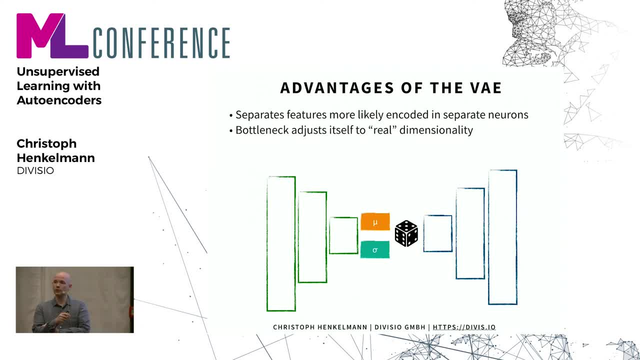 if it just needs 20 neurons, but it has 30, it will not use 10 of them, So 10 of the neurons will be dead. They won't produce any output in the generator, And that way it's much easier. 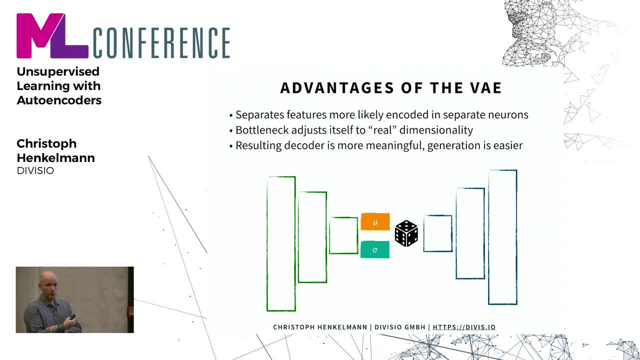 to build an autoencoder that works. You can look at the autoencoder and determine how many dimensions are actually used, And then you know the dimensionality of your problems. Also, it means that the variational autoencoder doesn't overfit. It doesn't overfit so strongly. 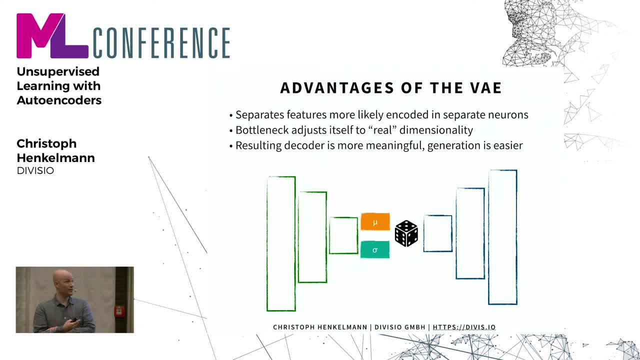 Because if you give it too many bottleneck neurons, it will simply not use them. That's super cool And the generation results are much more meaningful And the latent vector is much more meaningful, which in turn means that transfer training will produce better results. 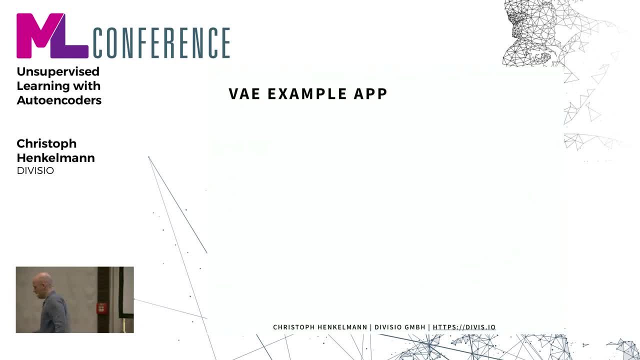 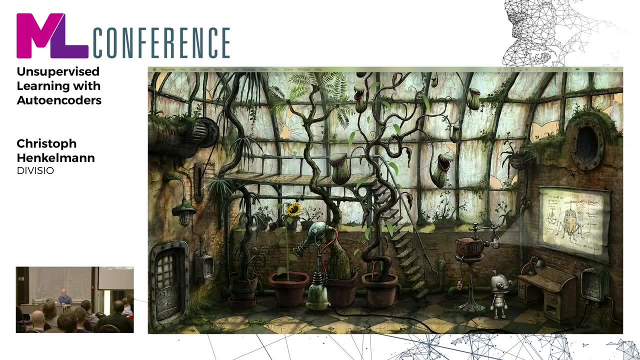 Okay, But I think what's more useful here is we actually, if you look at an application that does that. it's not perfect, but I hope it will help you get the idea. I have to quickly change the. I have to quickly change the way the display works. 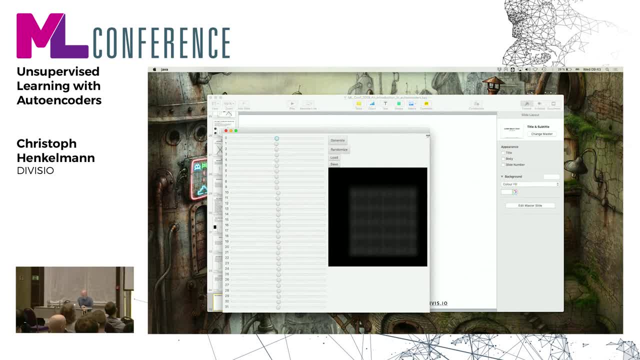 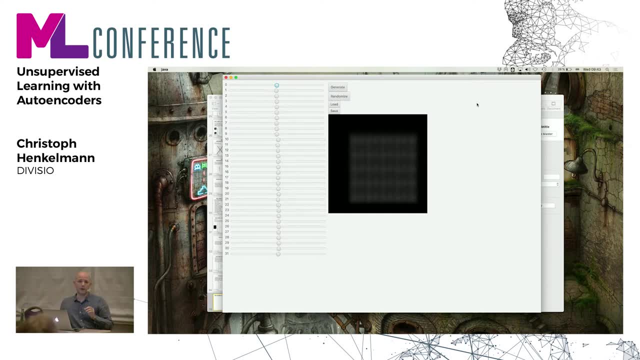 One second. So what I have here- I hope it's large enough to see it- is an application that uses a pre-trained autoencoder, a variational autoencoder, to generate MNIST images. Here you have the generated MNIST image. 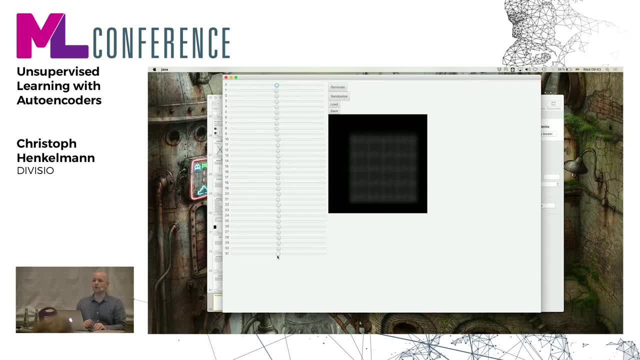 And here you have 32 sliders that control the bottleneck neuron's values, And what I can do now is randomize and we will see. those are not really numbers, but you see halfway decent structures And, for example, now I have what I would say: 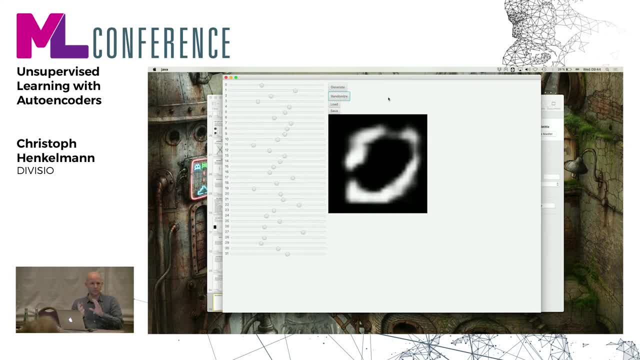 is a pretty nice zero. It's a bit smooshy, but we would. I think everybody would agree that this is a zero right? So what I can do now is I can explore. we have one point in latent space. This zero is actually a 32 dimensional vector. 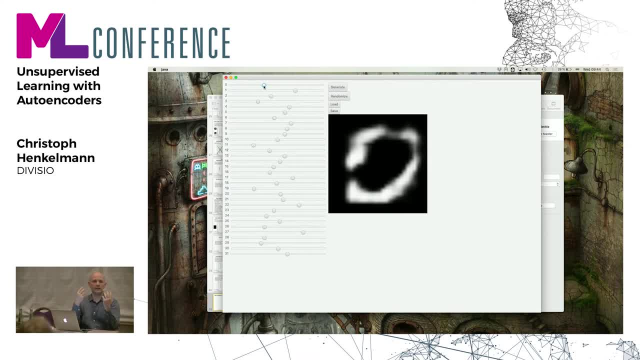 that is turned into an image. And now what we can do is we can explore the surroundings of this point by interactively, by just changing the slider. So we see this: with this slider we can move the zero more towards a nine. 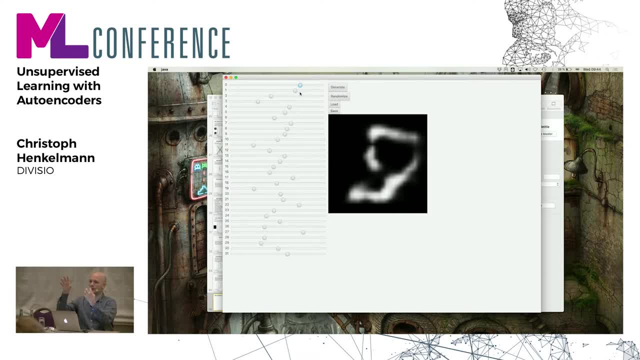 So we know, in latent space, in this dimension, zero and nine are closely, are placed more closely, So we could generate more of a nine here. Let's try and make this nine a bit better. So here, some of these are not completely understandable. 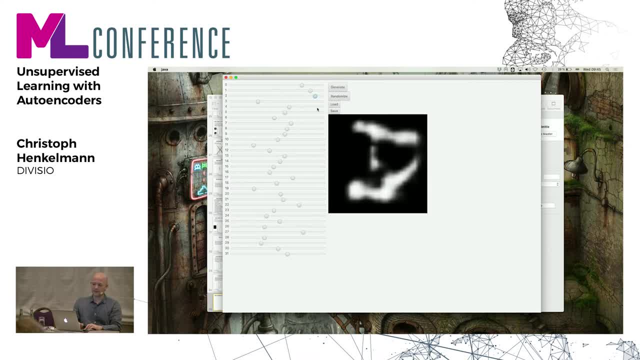 from a human perspective. but we see that this one creates lines at the top and the bottom. That might be useful if we want to build a seven, And here, yeah, some of them- not each dimension- is really useful, but here you see something else. 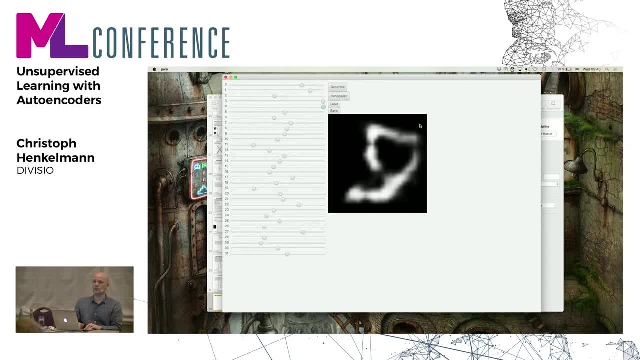 See what happens here. Nothing. This is one dimension. the variational autoencoder chose not to use. It said: well, I don't need this, So this neuron doesn't do anything useful, so we can turn it down Here. this one is a bit more useful. 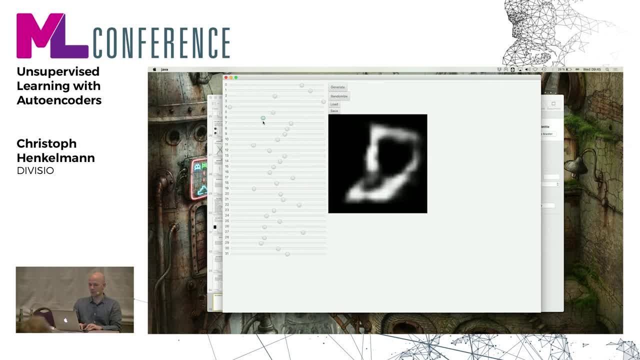 We can see this one does something useful And we can do this. ah, here we move more towards a zero again. Ah, but this: you see how this closes the upper right loop. So this dimension, at this position, changes to the upper right loop of the nine. 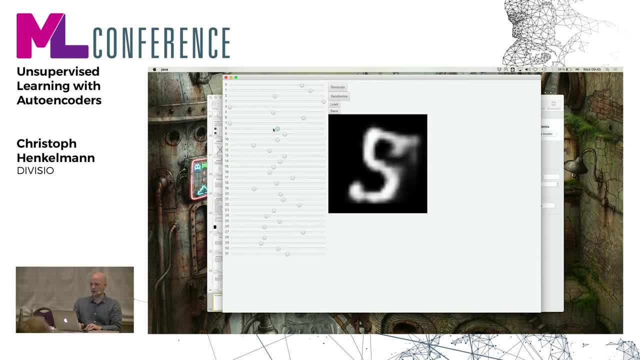 And you can here again: we have a dead dimension. And with this, yeah, each of them- sometimes it takes some time to find out. It's just fun to explore your data that way, because that way you start to understand how the network. 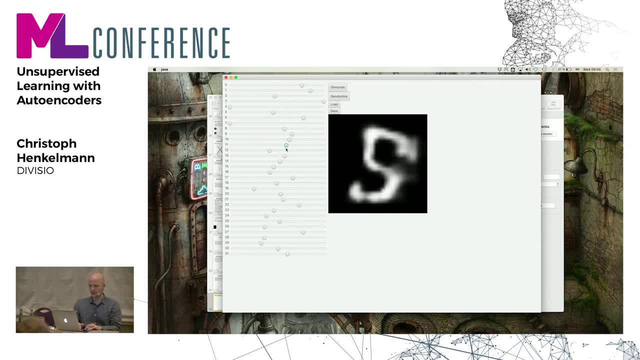 or you get at least a gut feeling of how the network works internally. Yeah, this is another dead one. Yeah, that way you can explore what the variational autoencoder learned. So you see, just after a few steps, I think this is a pretty passable nine. 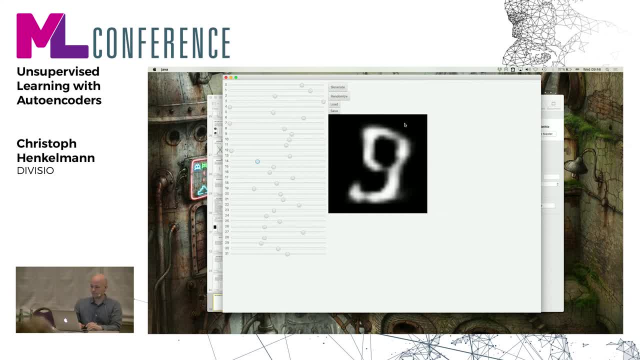 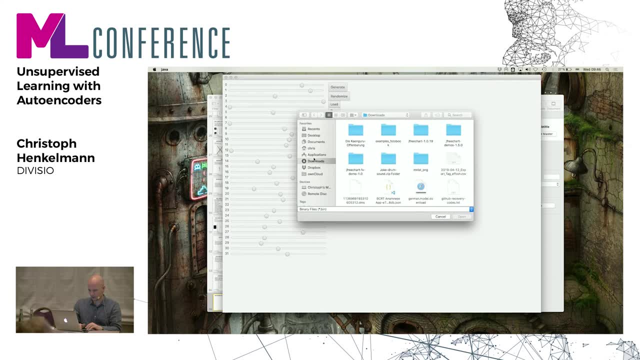 So we have learned how to encode a. nine here. Yeah, the funny thing is, I'll just load a. I created some examples beforehand: Ah, mm-hmm, mm-hmm, mm-hmm, mm-hmm. one minute one else. 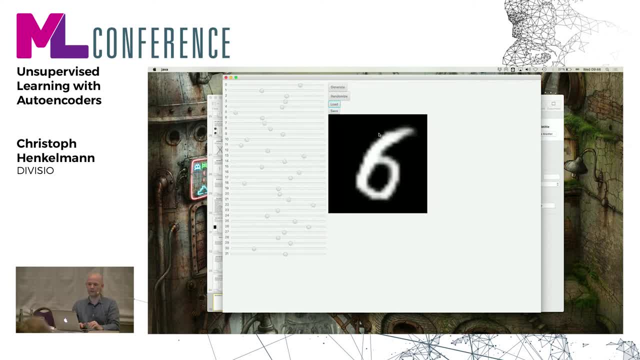 So here I generated a six. This is a very nice six. What you? ah? I thought it saved the dead dimensions. Before the talk, I actually tried out this app and after a few minutes of trial and error I found out that there are about 10 dead neurons. 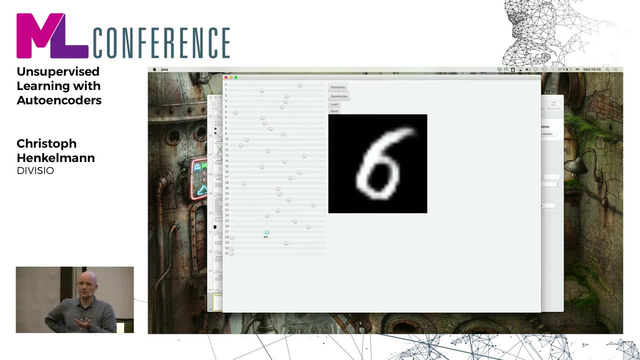 Remember earlier I said that MNIST has about a latent space size of 20. How do I know? Because I actually looked at the latent space and could find out. So this is really useful for complex problems that you can actually look at the encoding the neural network has internally. 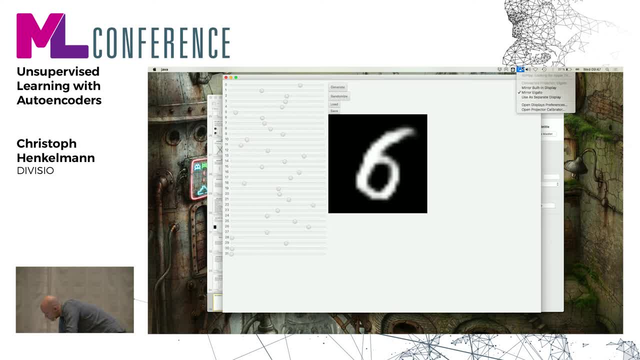 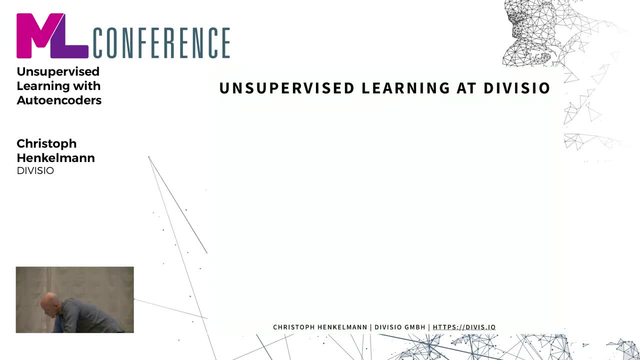 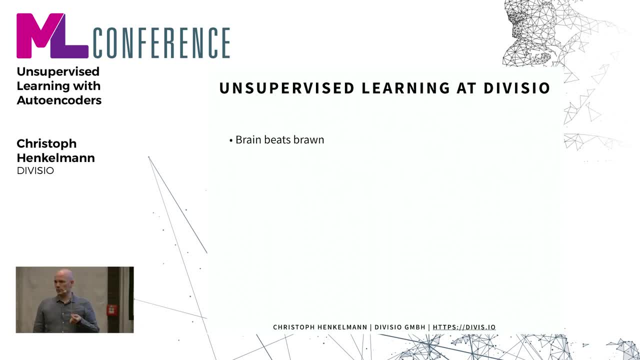 instead of just throwing more and more labeled data at our problem. It helps us understand the problem more, and I kind of like that For us, we are smaller player and this kind of stuff allows us to do things that would be normally beyond our reach.